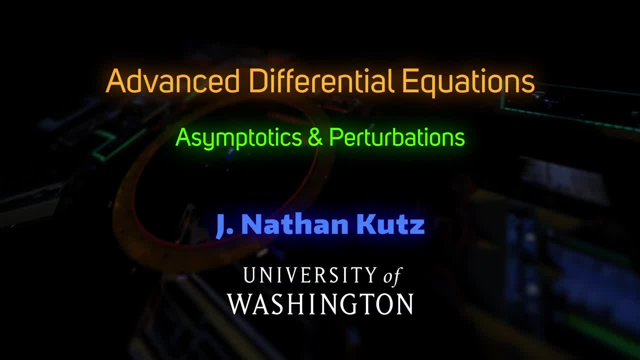 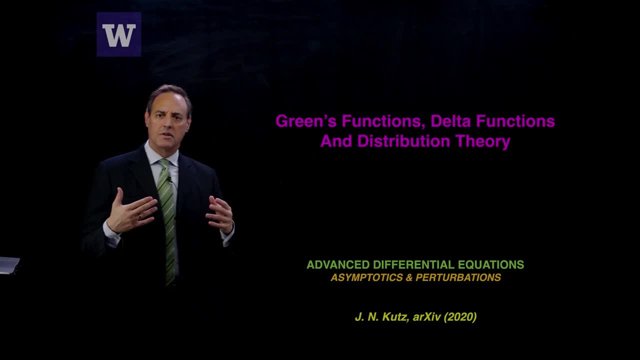 So we're going to change gears a little bit to talk about solving LU- because F-type problems, and these are typically boundary value problems- and we're going to switch to solving them using what's called the Green's function. Now the Green's function introduces several new concepts and 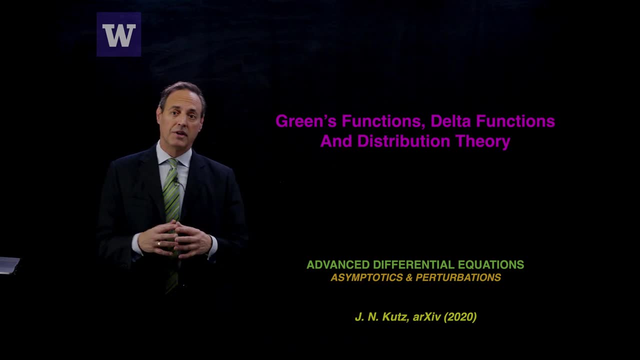 specifically introduces this idea of distribution theory and direct delta functions and or impulses to a differential equation. So this is a really important concept and we have to think about how do we want to define these objects, because we're going to use this to construct our Green's. 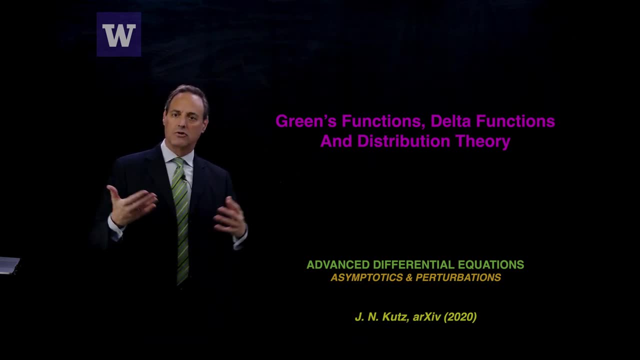 functions, which are also known as the fundamental solution to the differential equation. So it's a very powerful tool. If you can compute a Green's function for these problems. it gives you this ability to compute any solution for any right-hand side function. F in LU equal to F. 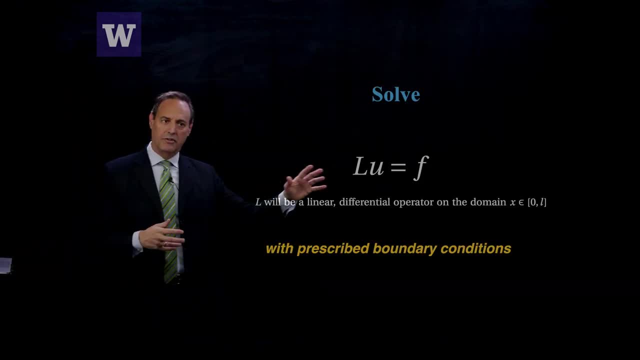 So let's go ahead and do that. So let's talk about the construction of this. Remember, this is what we're trying to solve here: LU equal to F, And typically this is defined on some domain 0 to L, okay, and L is a linear differential operator. 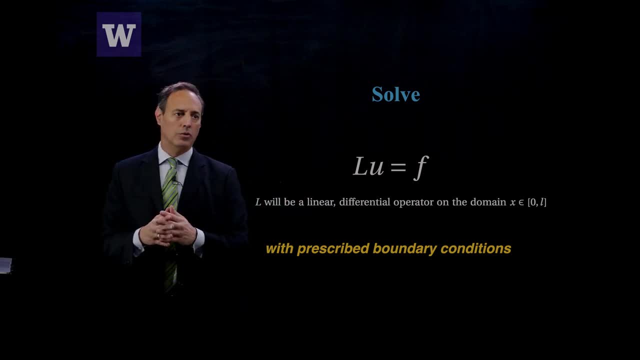 So what we want to do is decide: how do we find solutions U given a forcing function F and given this linear differential operator L, and how do we prescribe and construct solutions U of X in some kind of pragmatic and disciplined fashion? So we have that plus documentary conditions. 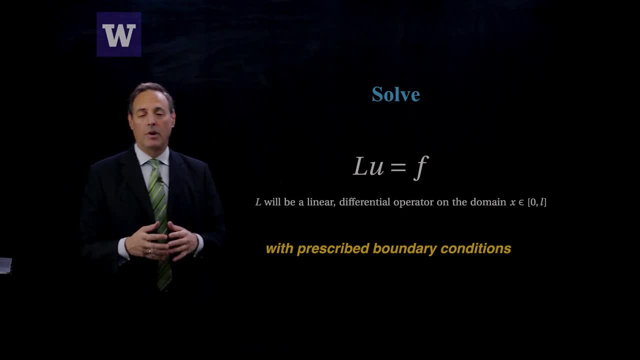 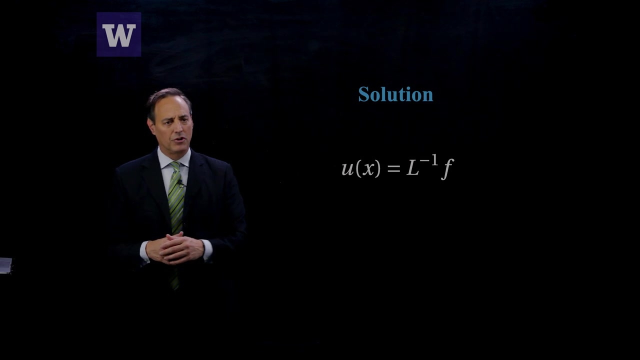 What we learned previously is: you can use this. you can find actually the eigenfunctions and eigenvalues of L, and then you can do an eigenfunction expansion, which is one of the solution types you could use for this. Ultimately, what that resulted in was some kind of approximation for the inverse of that operator. 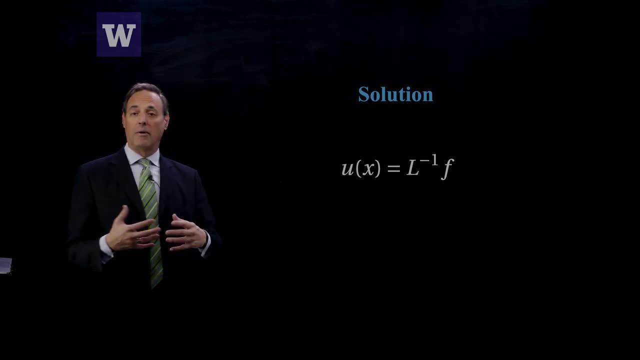 So this is very much like AX equal to B, but now it's a infinite dimensional function, space. and so when you solve L equal to F, there's this concept of finding the inverse of the operator L, which is L minus 1, okay, And so we want to find the equivalent of that, or the equivalent of 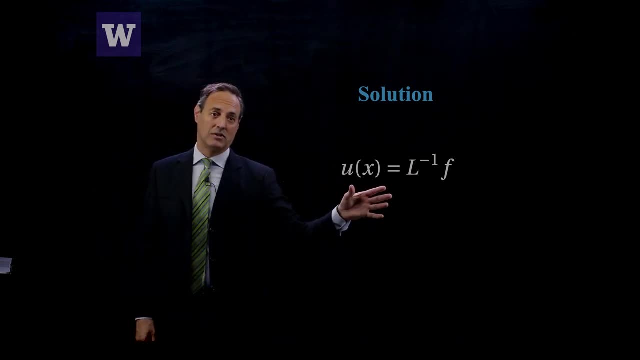 A inverse of a matrix to compute solutions such as this. So the Green's function is going to go a long way towards answering this question, which is: how do we compute that inverse? Okay, so, before we get started on the Green's function, 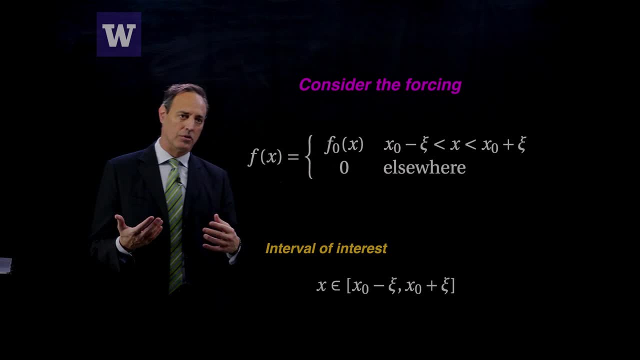 there's an important conceptual piece that needs to be introduced. So consider the forcing having the following form: Suppose this F of x. here it's 0 everywhere, except it takes on some functional form: F naught, x around x naught. So there is some point. on the interval 0 to L, 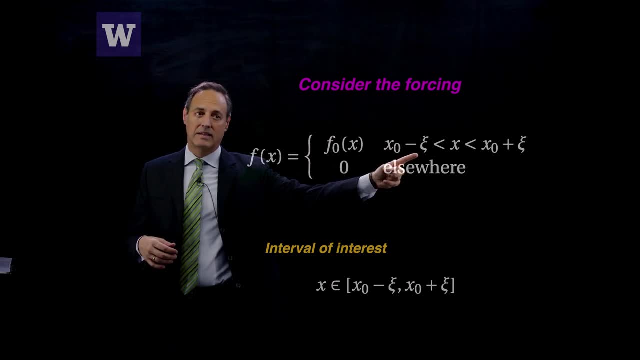 x naught and in a neighborhood of this, defined by this xi. so xi to the right and xi to the left. at that point I define the function F and it's 0 everywhere else. So the only interval of interest for us. 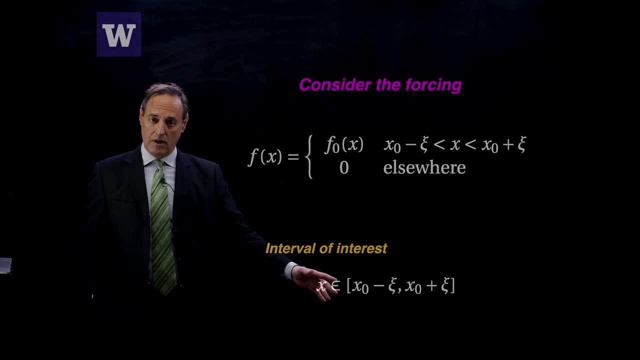 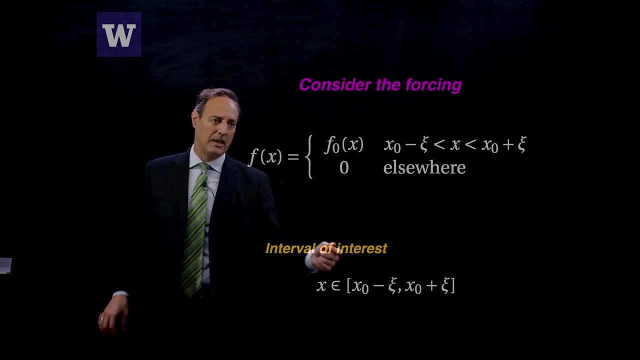 where F is non-zero is here in this small interval. Okay, I haven't said it's small, but that's ultimately what we're going to do. is we're going to make the interval small by picking xi to be small? Okay, so this is going to be our forcing. 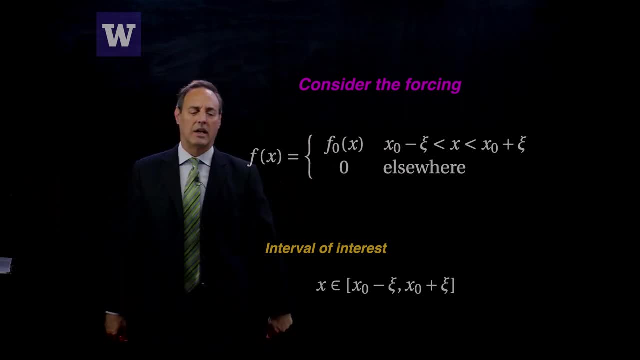 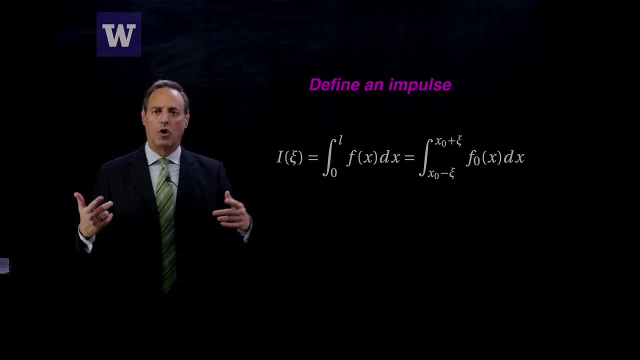 0 everywhere- small region where there is something interesting happening. So this is going to be our forcing: 0 everywhere- small region where there is something interesting happening. So, with this concept in mind, we can define what is called an impulse. 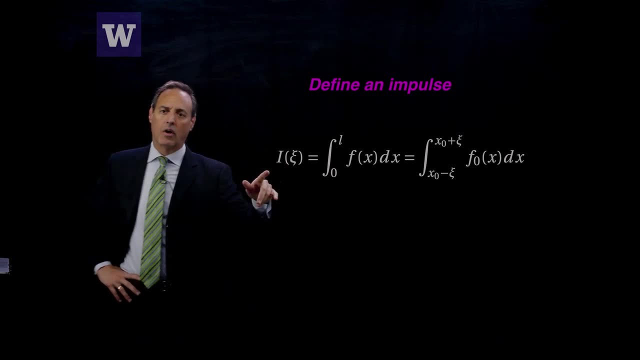 And what the impulse is going to be is going to be the integral of the function F of x over the range of interest for us. So, for instance, here the impulse is going to be a function of xi, because that's one of the parameters that I've picked there. You integrate over the domain of interest. 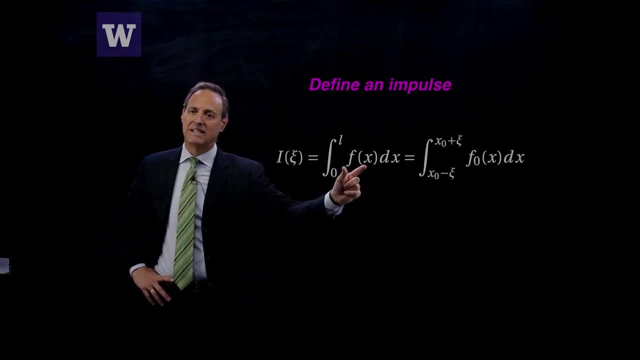 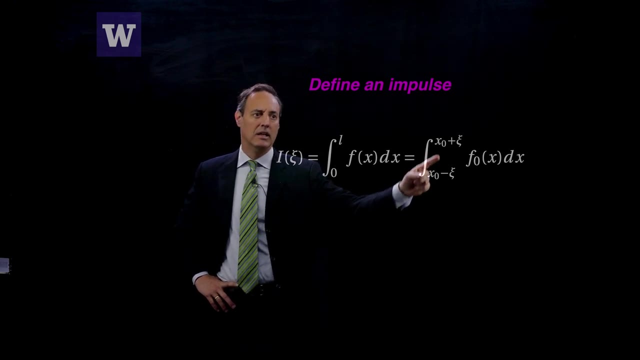 0 to L, F of x, dx. But remember, F of x is going to be zero everywhere aside from that small region around x0.. So we integrate from x0 minus xi to x0 plus xi F of x. So this is going to give us this concept of an. 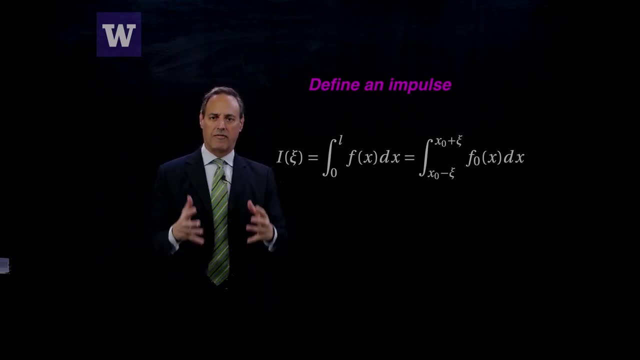 impulse. It is something that you integrate over this forcing function and the total area under the curve is the impulse. And this is going to be a really important concept for us because we're going to continue to develop along these ideas towards building out this Green's function idea. 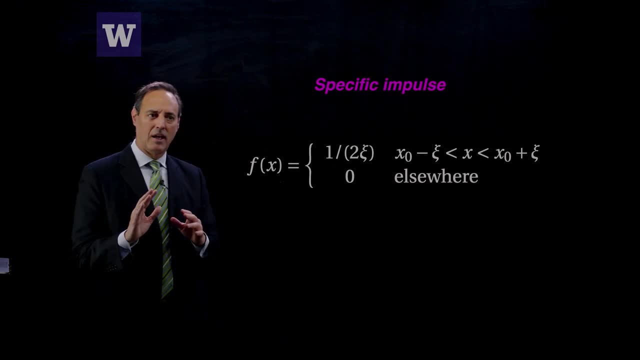 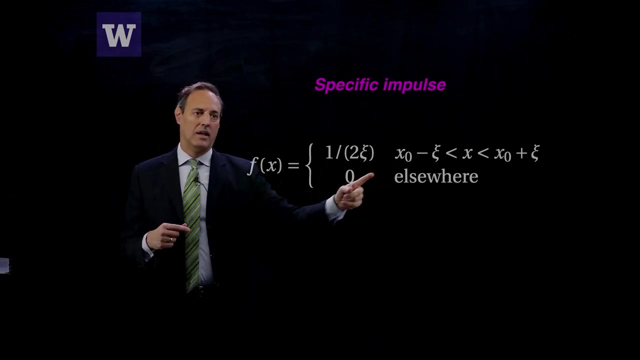 So let me give you a very specific impulse and I'll show you why it's such a nice one to consider initially for us. So the function F of x will have a height of 1 over 2, xi in this interval and 0 everywhere. 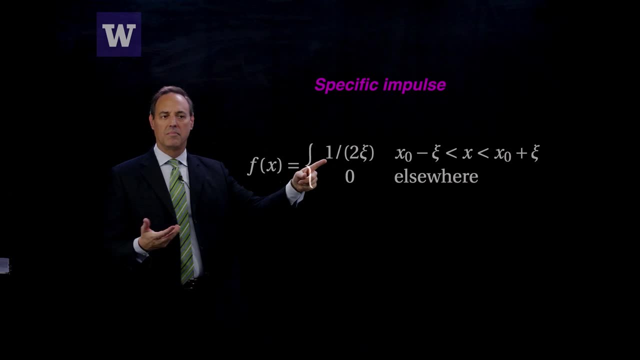 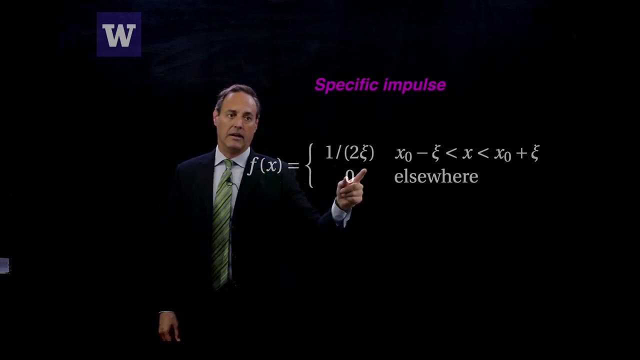 else. So I've just made this a constant, but a constant that depends upon xi, In other words the width of the interval I'm looking at. In fact, the width of this interval is 2 xi. the height of this interval is 1 over 2 xi. 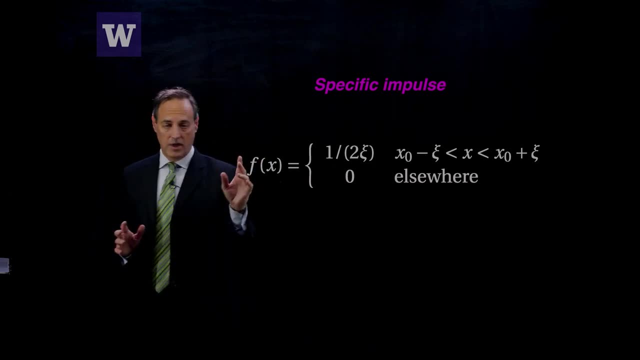 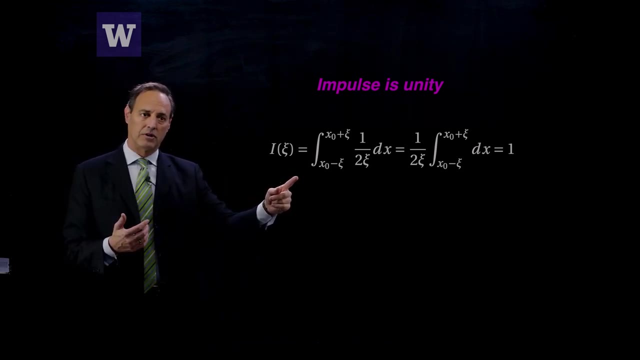 So this is a really nice impulse, or specific impulse, because what we're going to do is be able to compute the impulse function of this here, And if we find the impulse function of this, I integrate from x0 minus xi to x0 plus xi. 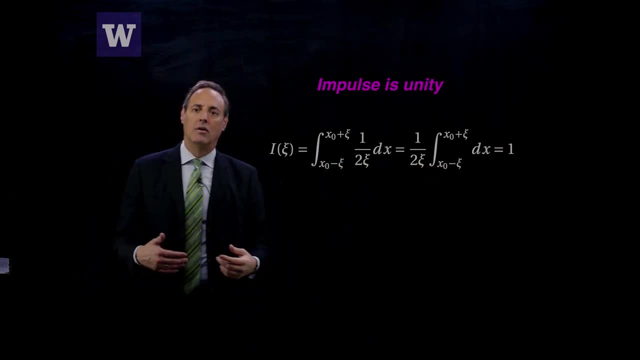 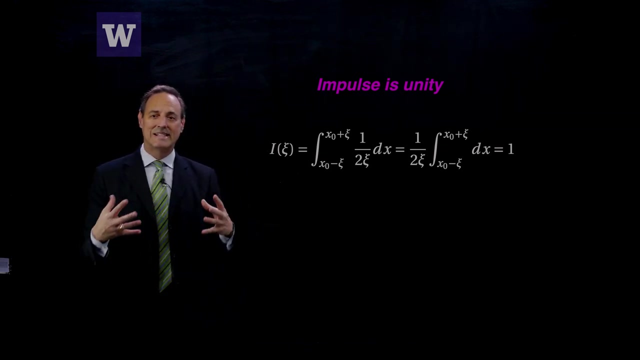 So you have 1 over 2, xi, dx, and this is equal to 1.. So this specific function, the total impulse, is unity, And this is going to be an important class for us, because what we're going to do now is we're going to start shrinking c towards 0.. 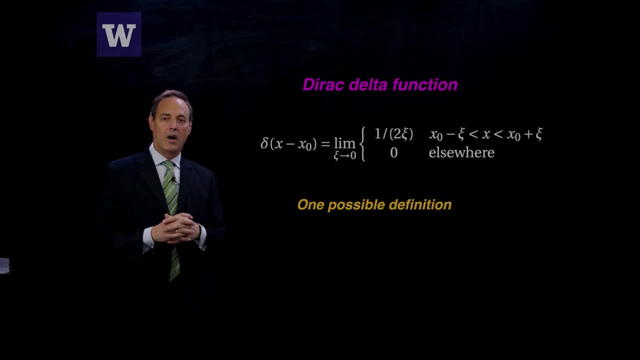 So, in fact, when we do that, this is what's called the Dirac delta function. It's defined by here: delta x minus x0.. You may have seen this, in fact, when considering Laplace transforms for solving ODEs, It shows up in a lot of places. 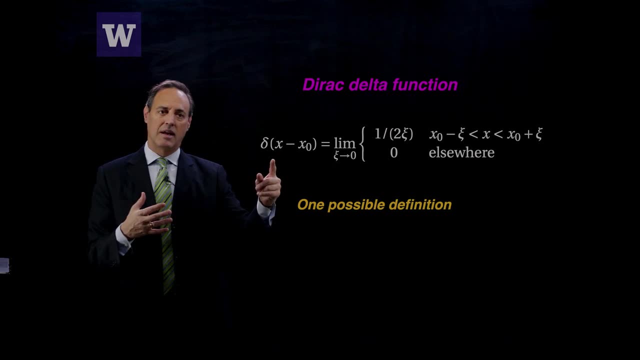 across physics, But here is its definition. This definition of the Dirac delta function is the limit xi goes to 0 of that function. So what's ended up happening is this function is 0 everywhere, except for this small region where type 1 of 2 xi. 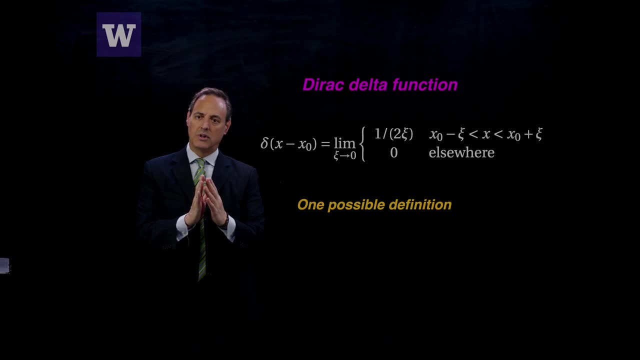 And then you make, the xi goes towards 0. So the region shrinks, but the height goes towards infinity, in such a way that the impulse, in other words the integral of it, is always 1.. Okay, By the way, this is only 1.. 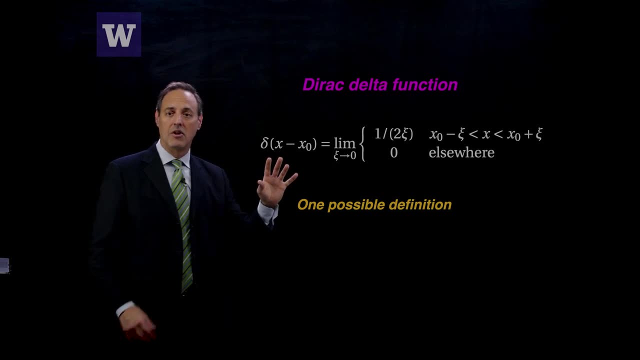 There are one possible definition of the Dirac delta function. There are others. In fact, there's a whole class of what are called distribution theory, which outlines a number of Dirac delta sequence functions that produce the same kind of behavior, which is they get smaller and smaller in the interval. height goes to infinity, but in such a way. 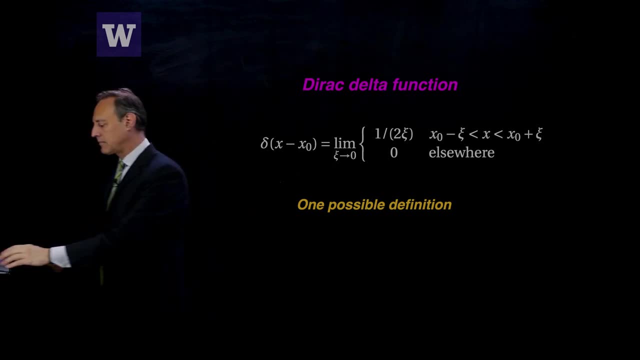 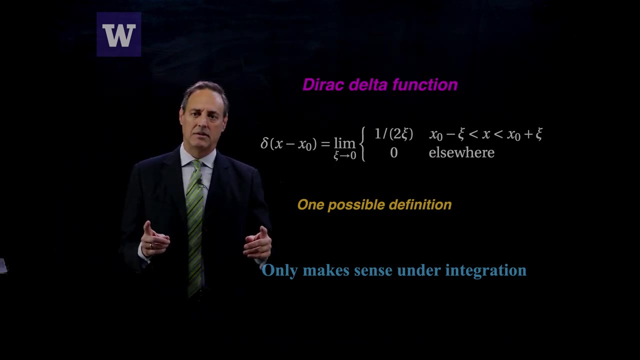 that the area under the curve is 1.. In fact, one thing to point out here is this: This is not a function in the standard sense, And this is why we have to introduce this concept that was called distribution theory, which I won't talk too much about. 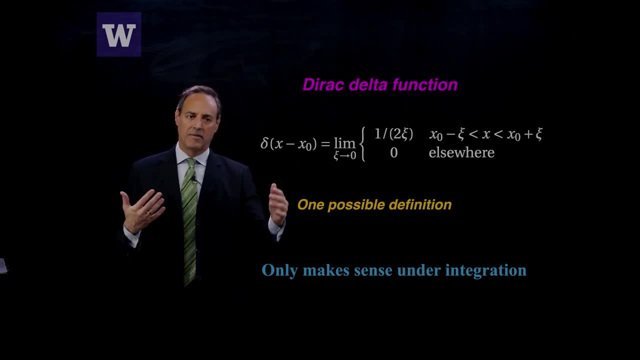 But basically it's a generalization of a function that only makes sense under integration because the amplitude of this is going towards infinity. So it's 0 everywhere and infinity in one spot, But from an integral point of view there is no problem. 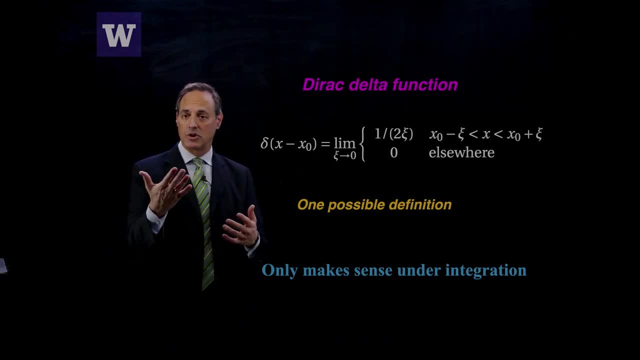 You can integrate over this, and it's always a finite number, which is 1.. So we have to multiply. You modify our thinking about what function spaces are, and this is what distribution theory does. By the way, I did say, this is not unique. 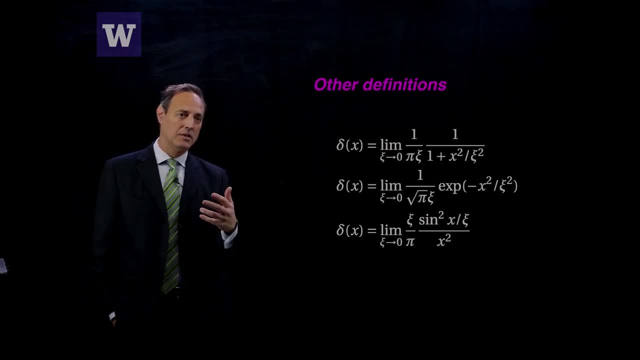 This was just one delta function sequence. There are others. Here's for instance three others here. You can take something like a Gaussian here. This is a sinc-type function and this is a 1 over 1 plus x squared, so like a Lorentzian-type. 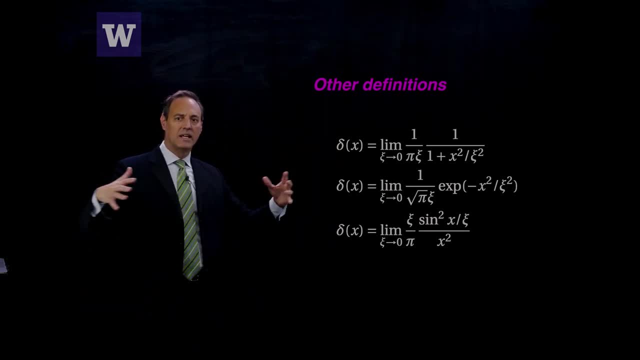 function. So these are different sequences that, as you take, c goes to 0, they all kind of produce the same kind of limiting behavior. What they do is they live on a smaller and smaller range. The height goes to infinity. so you're squeezing this function in. 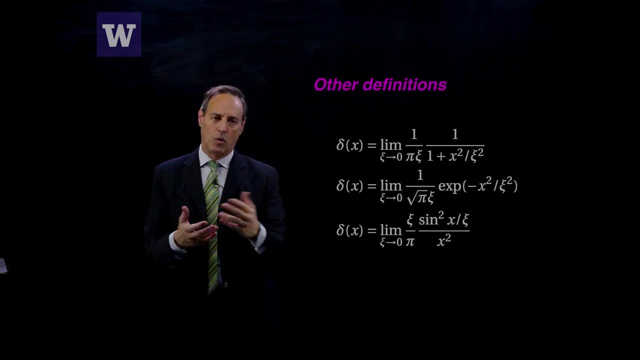 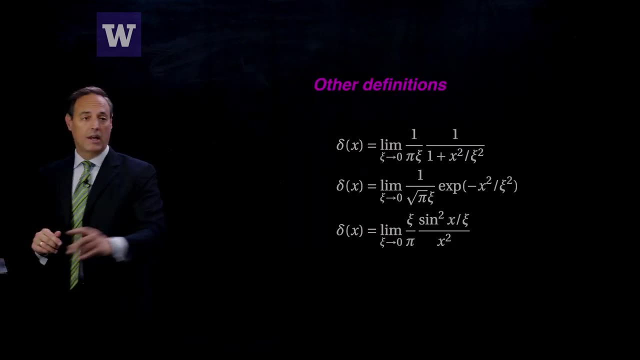 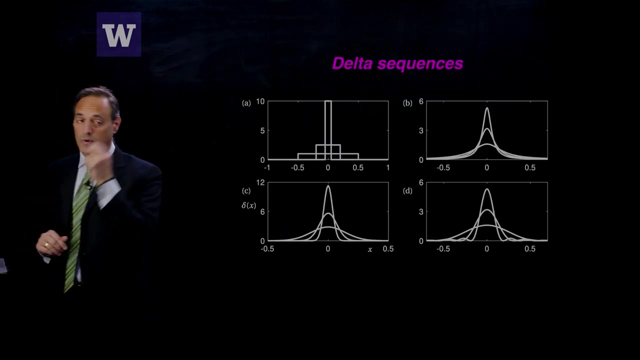 Height goes to infinity, but the area under the curve is 1.. So let me show you some pictures of these, and here they are. So what I'm plotting here is these three delta function sequences, along with the first one I introduced, which is the one right up here. 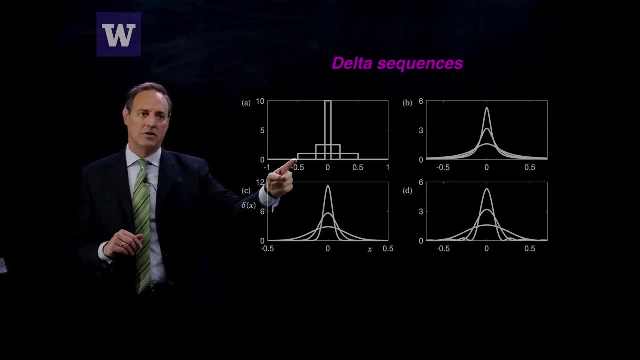 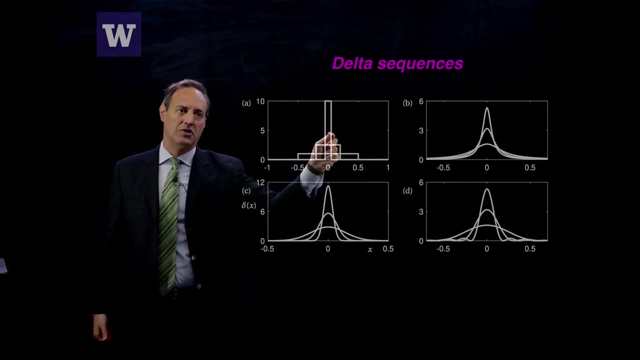 So notice what happens as c gets smaller and smaller. It starts here. I'm squeezing this together and notice that it's getting taller and taller, but the area under the curve of all these is always 1.. And what the delta function is is, as I squeeze it towards a width of 0, this goes to a height. 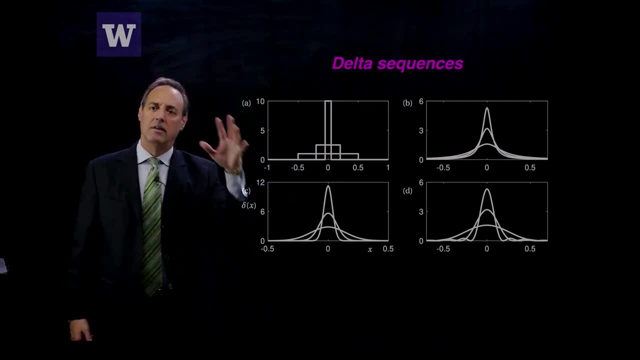 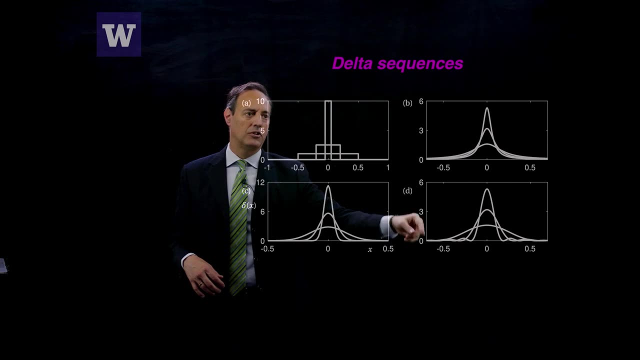 of infinity, but in such a way that the impulse or the integral of it remains. 1.. Here are some of the other functions and what they look like. Here's the sinc function, You have the Gaussian and then you have the Lorentzian type structure. 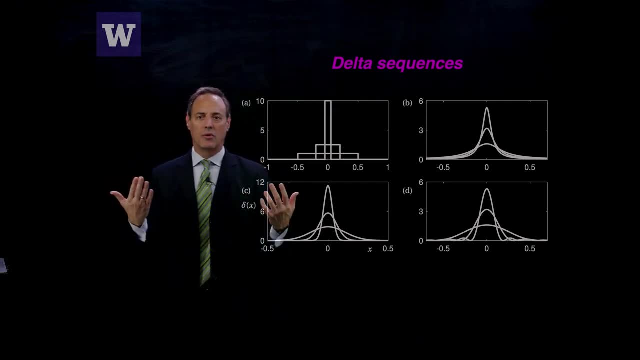 So these are different definitions of a delta function. The easiest one to work with, of course, is the one I just showed you, which is this here, because when we're going to play around with it and show some of its properties, this is: 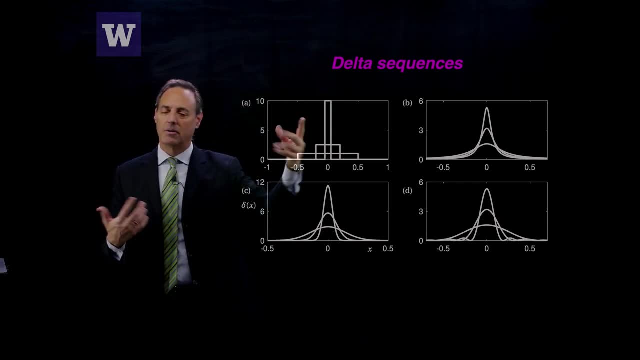 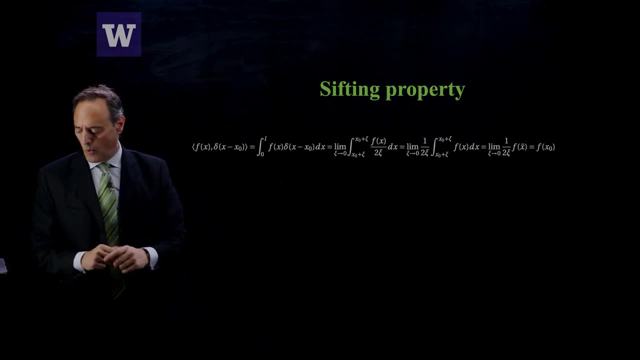 so nice because it's 0 everywhere and then it's only non-zero in a very small place. So we'll stick to that one for now. So why would we introduce this function? Well, this function is going to be really important Because it's going to have what it's called a sifting property. 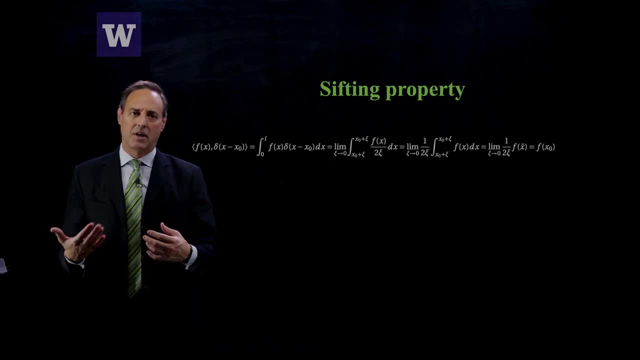 And in fact this is the most important property of the delta function. So what I'm going to do is take the function, some function f of x right here and then take its inner product. with this delta function, Now the inner product is an integral. 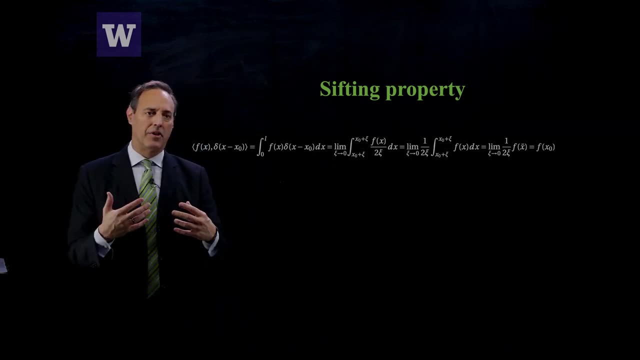 As such, this impulse function or distribution theory tells me that this delta function makes sense in the context, in the integral, And so this is going to make sense for me here: to take a function f, integrate it against the delta function. 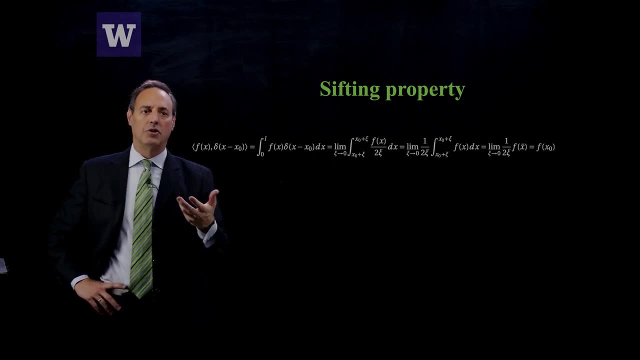 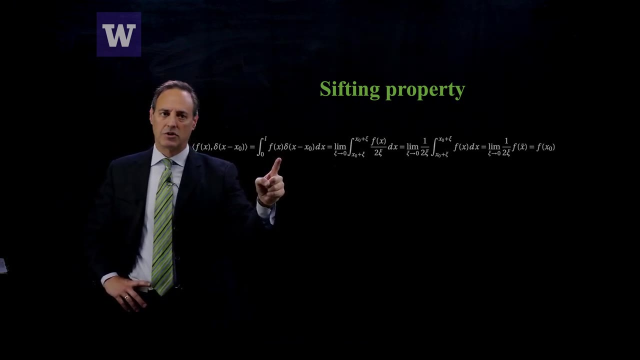 and one of the questions you ask is: well, what is the result of that integral? So if I do this- and now I go ahead and take this here- here's the integral of this thing. So it's just f of x integrated against the delta function. 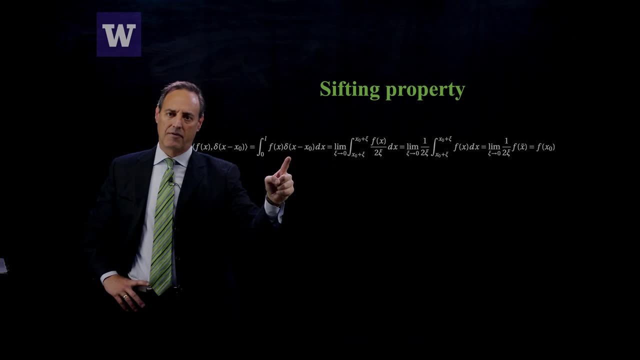 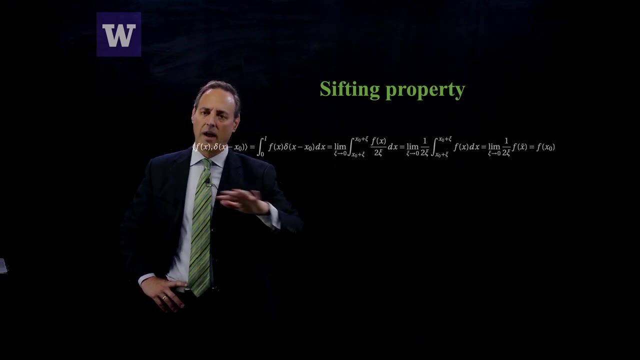 And now what I'm going to do, for this delta function is put in the definition that I had before, which is: it's the limit. c goes to 0. This thing, this delta function, is 0 everywhere, except around between x-naught minus xc to x-naught plus xc. 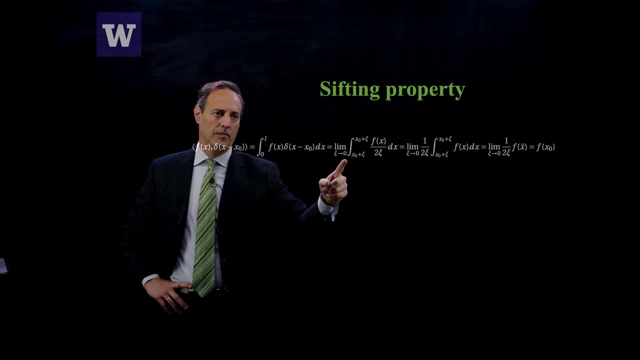 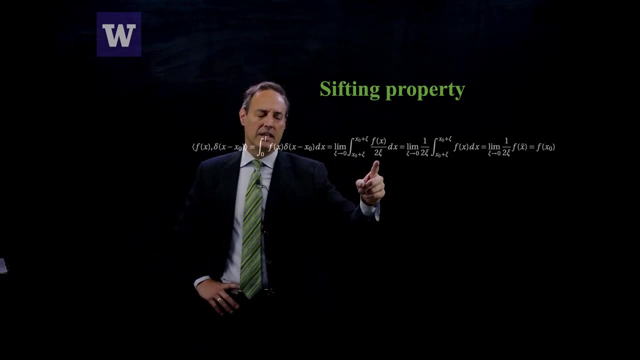 so that's why now this integral is in that limited regime f of x, the height is 1 over 2xc dx, And then what you can do is you can use your mean value theorem or you can actually pull out this 1 over 2xc. 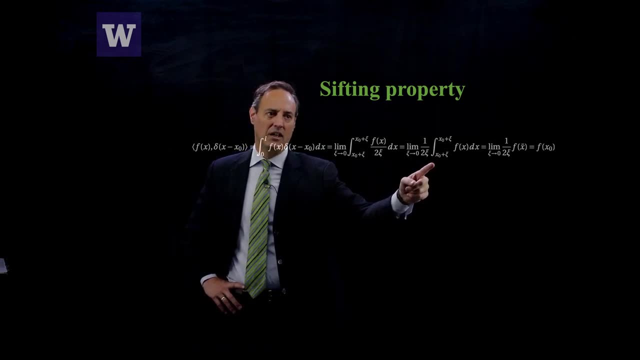 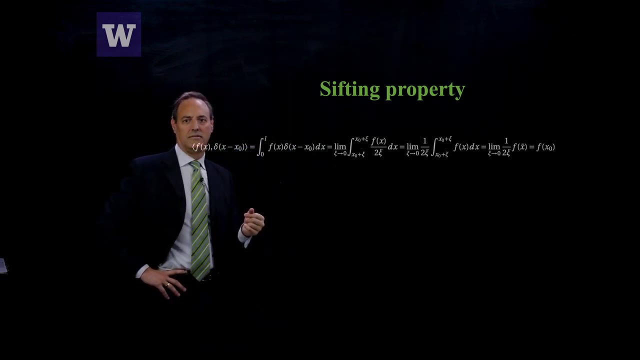 and now you use your mean value theorem and if you squeeze this c right, if you make c smaller and smaller and smaller, this thing here simply goes to f of x-naught. So that's it. So what this does is when you integrate any function, 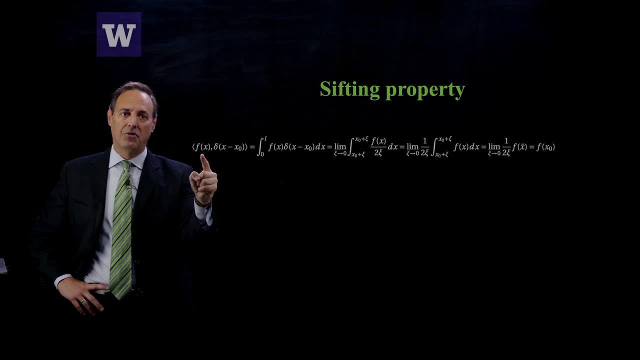 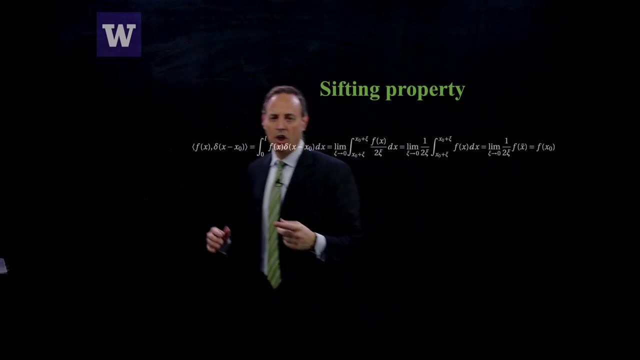 f of x against the delta function, it pulls out the value of that function at x-naught. That's exactly what we show here in that limit. So this is a sifting property. This delta function picks out wherever the delta function is placed. 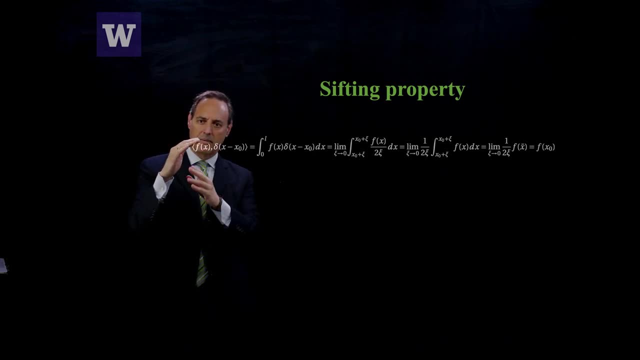 it picks out, under integration, the value against some other function, the value of that function at that point. And this is where we're going to make use of this for constructing our delta function solutions, or, sorry, for our Green's function solutions that we're going to use as fundamental solutions. 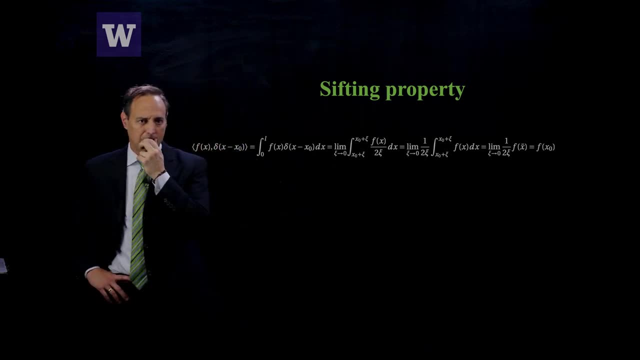 to L equals to f. Okay, so that's one problem, And you already start seeing that we are starting to work now with inner products And, just like eigenfunction expansions, everything's going to come down to taking inner products and showing how we can use them to our advantage. 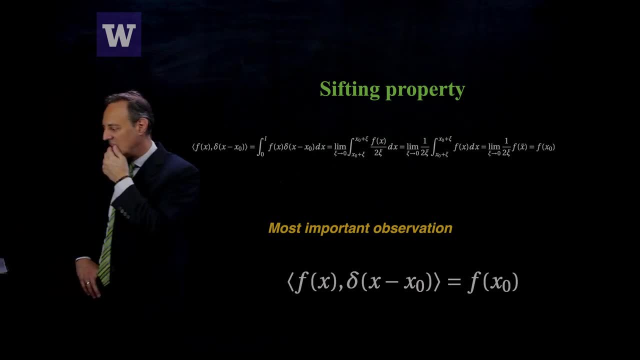 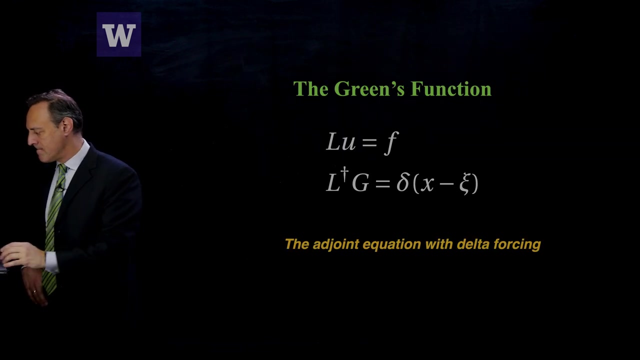 in solving for these problems. Okay, Okay. So there it is Just repeated the sifting property of the delta function. It just pulls out the value of the function wherever the delta function is acting. So now we're going to introduce the Green's function. 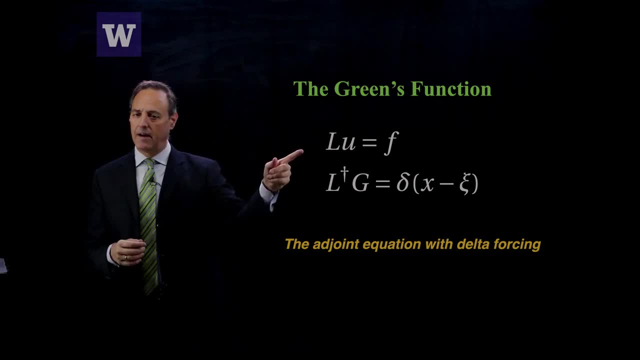 And here's what it is. So we're going to try to solve L equal to f. That's the problem we're trying to solve. And the Green's function satisfies the adjoint equation forced by the delta function. So you have L equal to f. 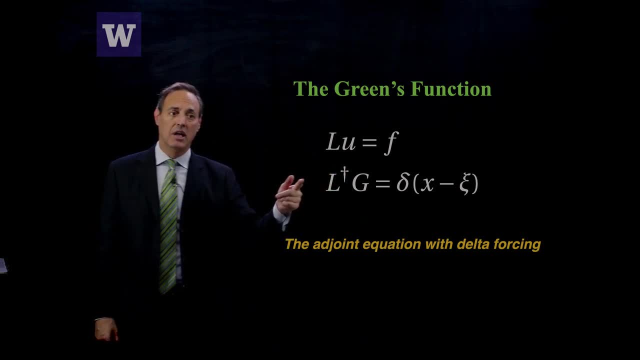 And then you have L dagger g equals to the delta function. Now we've already talked about how to construct the adjoint equations. So you would need to have the adjoint in its boundary conditions, And once you have that, you would go ahead and force. 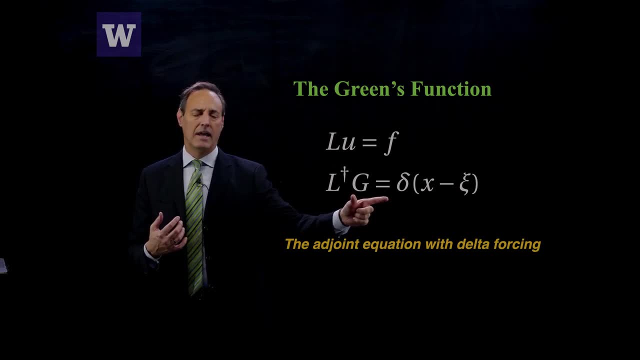 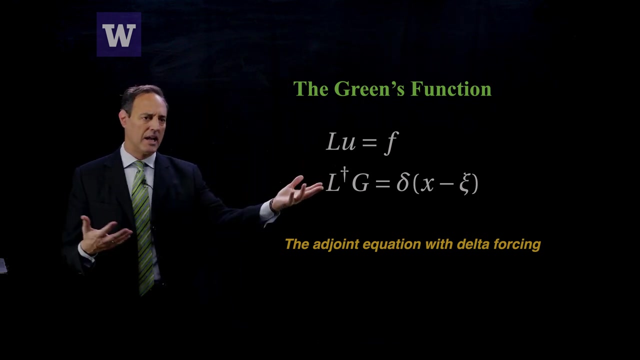 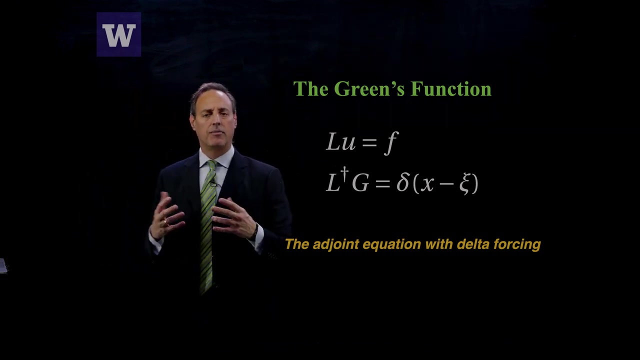 that with the delta function, And that is going to be now what we're going to use. That's how we construct the Green's function. Okay, So remember, if it's self-adjoint, that means the boundary condition, the. So what I'm going to show you is a, basically three. 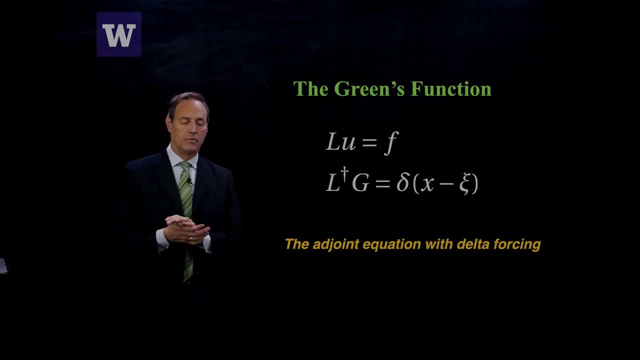 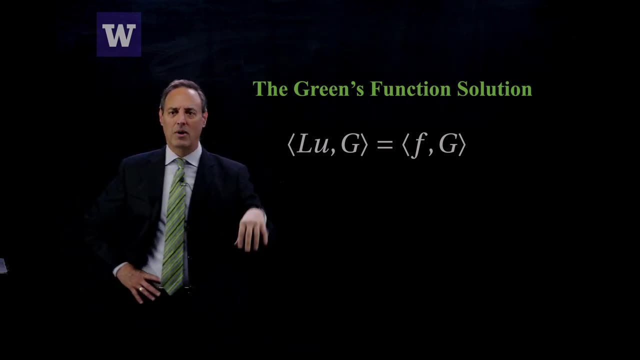 four line calculation which tells you exactly how the Green's function can be used to extract the fundamental solution for this problem or to give you a solution u So this you should be able to just do, And you should memorize this little set of calculations. 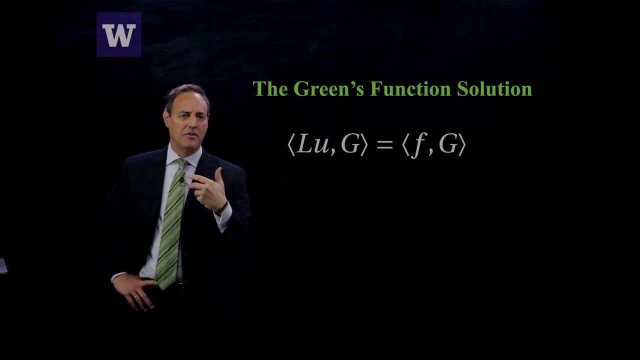 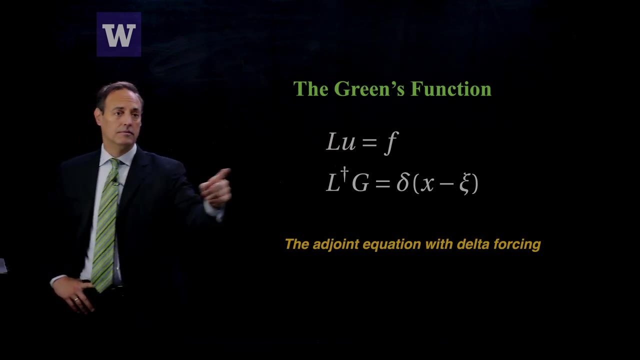 because they're just. this is everything, This is. once you understand these, this little three liner, then you know everything what the Green's function does. Recall here: this is where we're starting: L equal to f and the definition of the Green's function. 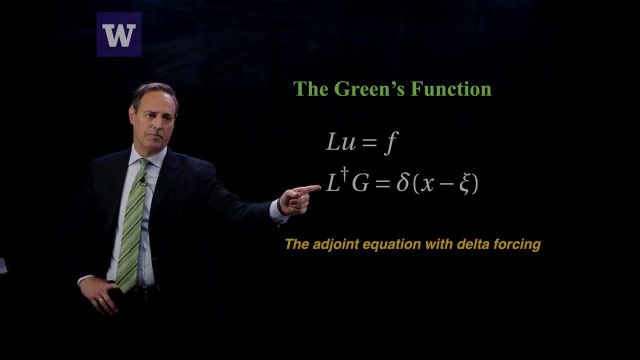 which is it satisfies the adjoint equation forced by the delta function. So what I'm going to do is take this equation here that I'm trying to solve, take its inner product with respect to the Green's function. So that's what I do here. So let's take the inner product on. 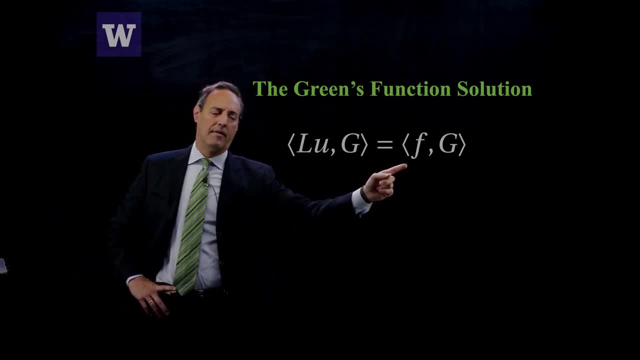 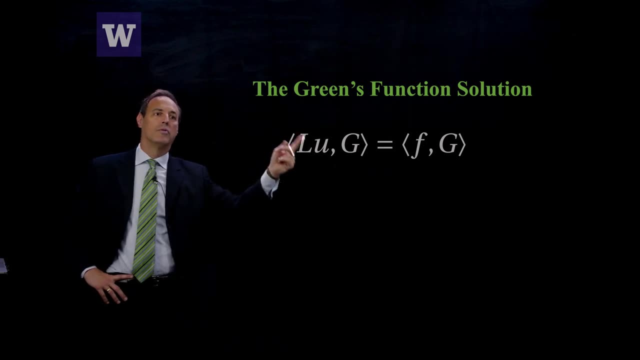 both sides. so L, U inner product with G, and then I have F inner product with G. Now what I normally do with this is I'm going to take this L then and say, well, let's move it over onto the G, right? So this is where I'm using my adjoint, So I move the L over. 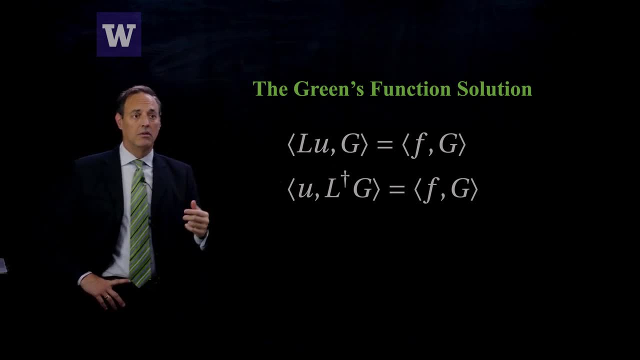 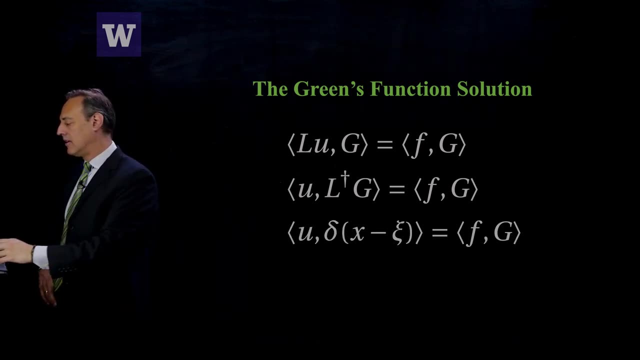 acting on U, now it's acting on G, So now I have L dagger G, But L dagger G is a delta function, right? That's the definition of the Green's function. It satisfies this equation where L dagger G is equal to this delta function. But I just showed you that if you integrate, 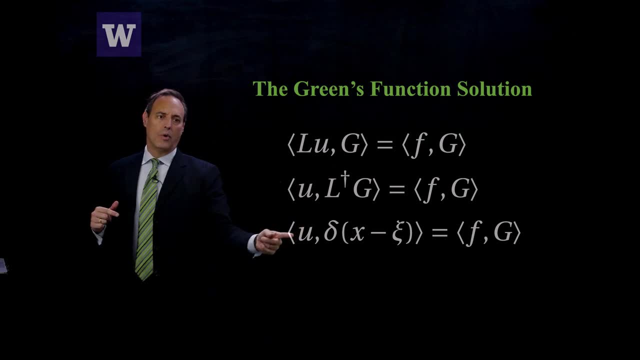 any function against the delta function. what it's going to do is have this sifting property and it's going to pull out the value of U at C, And that's it. There's your solution. U of C is equal to the inner product of F. 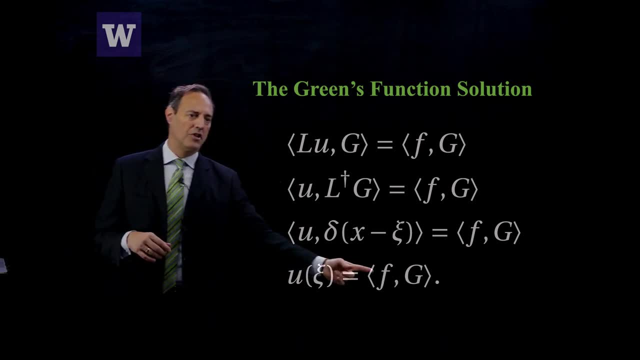 And then there's the solution of the integral of F against the Green's function G. So this is just some integral. So you just take your right hand side force thing F, and then you integrate it against the Green's function and you have the solution for the problem. 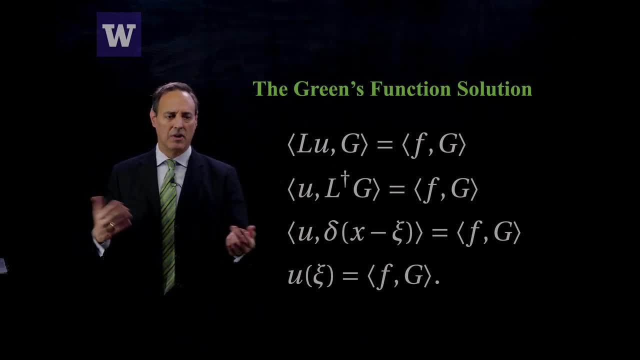 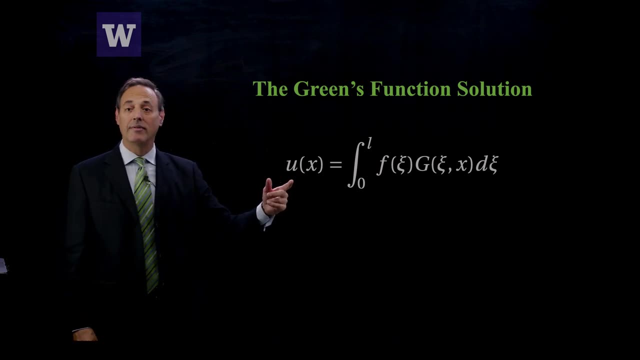 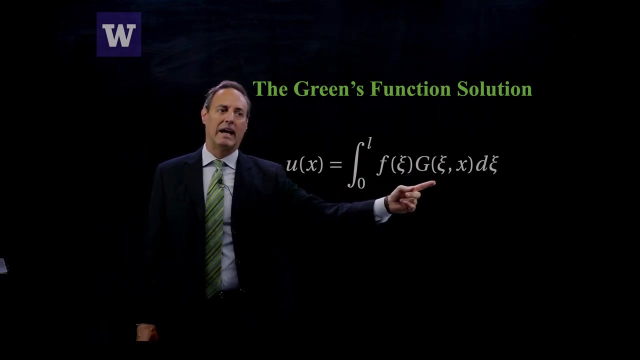 which is U here. Now C and X are dummy variables, So now I can just switch them one to the other And this is going to give me my final solution, which is just this here: U of X, my solution, f of xi, g of xi, x, d, xi. So g itself depends upon x. You can write it down: It's a dependency upon. 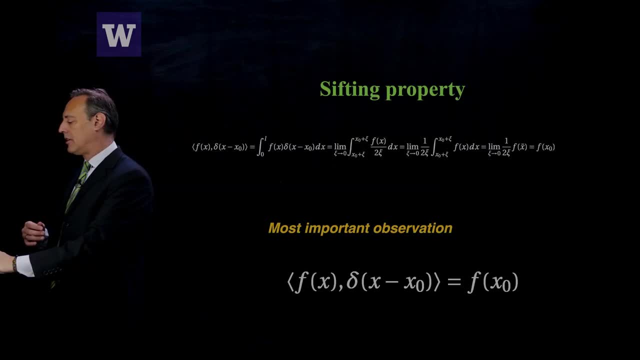 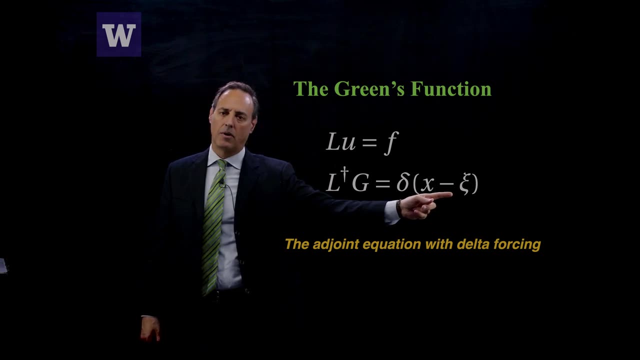 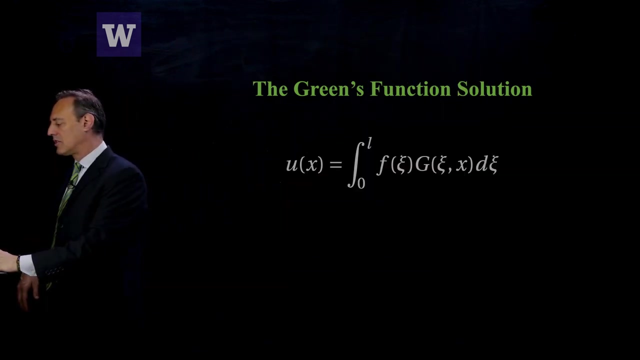 x and xi, because in fact here it is right there. So this is a function of g. but the solution, you know, it depends upon where the delta function forcing xi is. So you can think about g being a function of x and xi, and so now we switch those dependencies around to make it a function of xi. 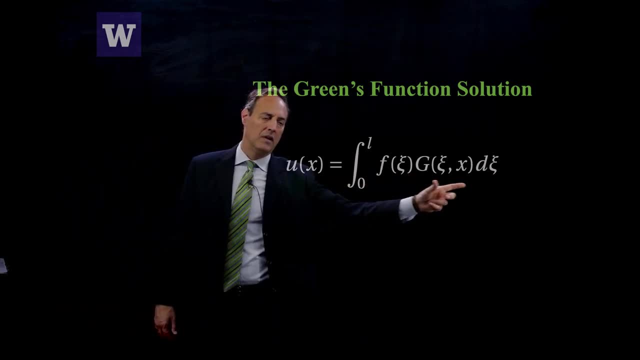 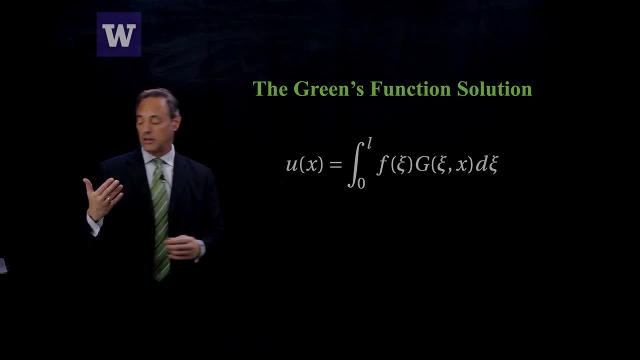 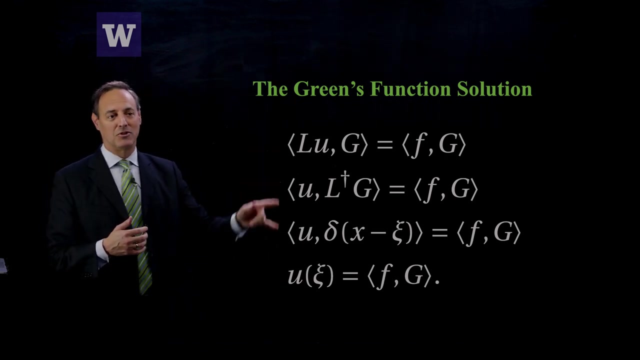 and x. These are just dummy variables, but I integrate this to find the solution u of x. Pretty nice, right? So this is a really important calculation. I highly recommend that. just memorize this. This is really important. You should be able to do this in your sleep. 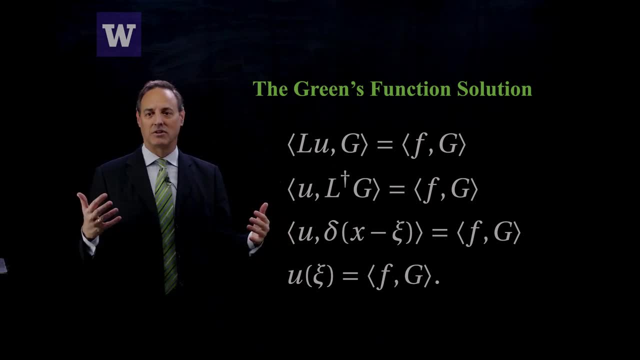 This is the main calculation of understanding what a Green's function does. So you have to just be able to do it And all it is is just take your problem, take the inner product with g, use the property sifting property of the delta function and you're done. This is this very elegant idea which 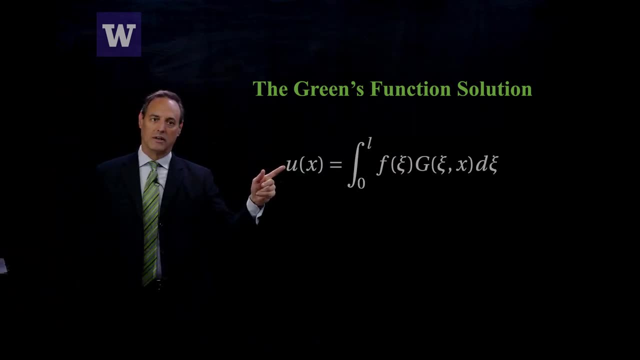 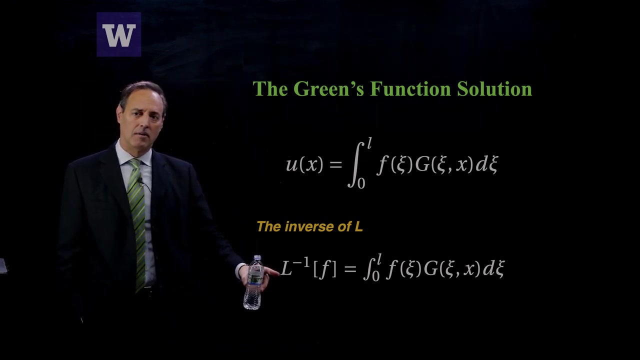 produces this solution right here. So I just need to calculate the Green's function and then you give me any f of x and I just integrate it and I've got the solution. So equivalent. essentially, what I've done is I've found the inverse right. So what this is telling you. 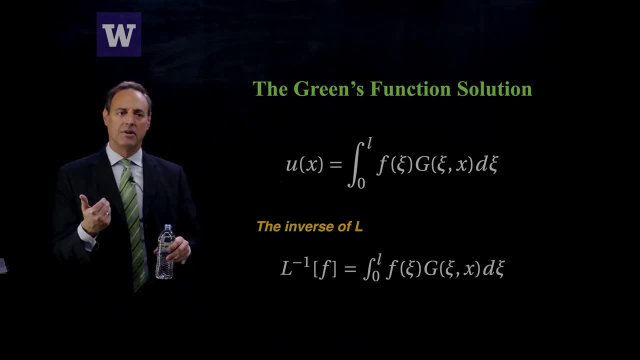 remember, L is a differential operator. The inverse of it should be some kind of integral, and this has a very nice representation of what that integral will look like. so it's in some sense it's giving you a nice concept of what the inverse should look like. 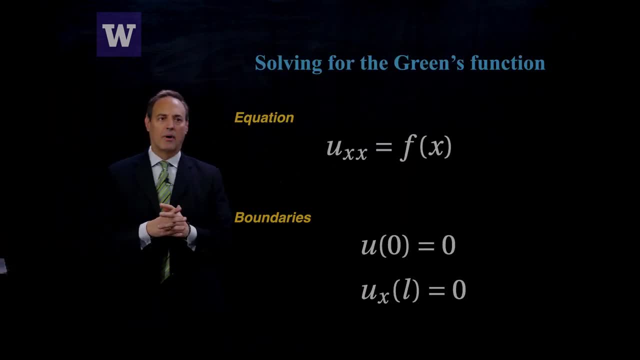 Okay, so let's go do a problem actually, just to show how this all works out. So I'm going to consider the following problem: u of x is equal to f of x with the following boundary conditions: It's pinned on the left and at exhaustive it's equal to f of x with the following boundary: conditions Pinned on the left and at outside. it's an actual branch And the diploma of this slide refers to a point v of x. There's little English words when I write down the Num total, So remember you take the problem if I have lots and lots and lots elements in the finding. 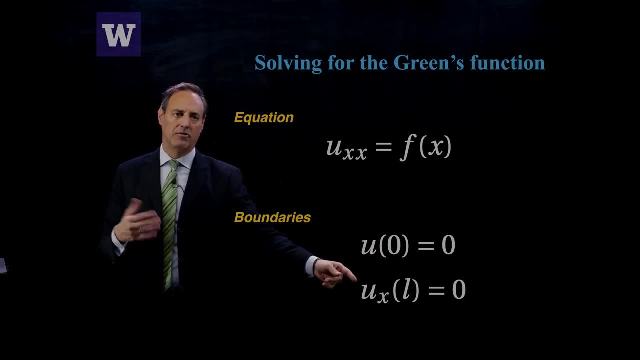 and at L the derivative is 0, so no flux on the right. So I want to find the Green's function for this, because then you give me any kind of new, different f of x's and I can just find the solution by integration. 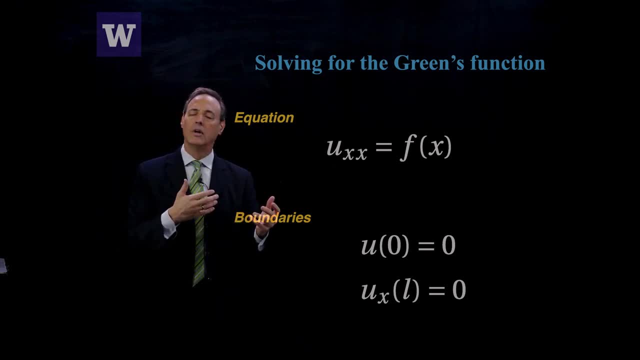 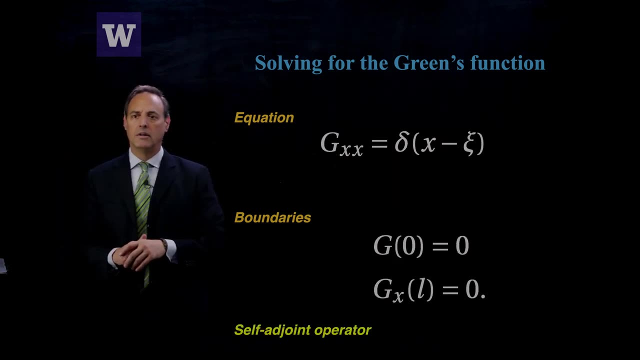 So I've already got the fundamental form of the solution I just have to give you. you just give me a new f and I can find a new solution. u. So let's consider the adjoint problem. It's a self-adjoint operator, so it's very nice. 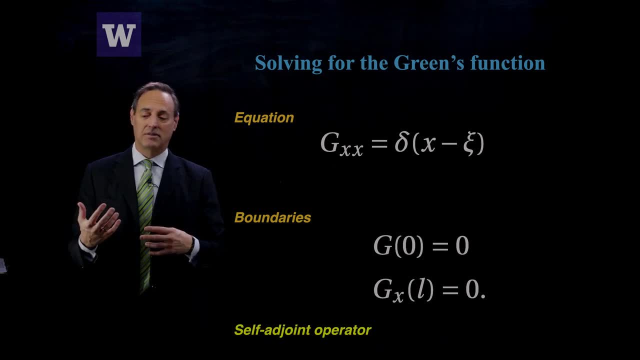 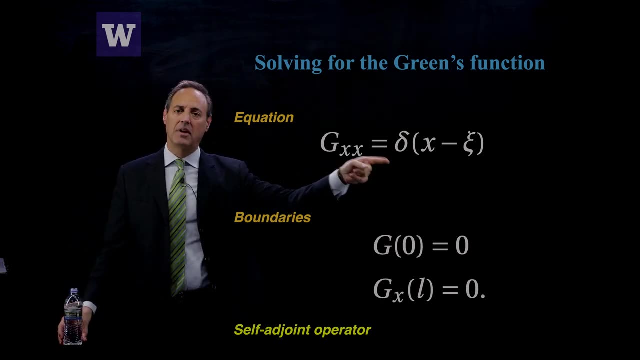 So the adjoint problem is the same as the original problem, right? So you have here g of x, but now, instead of an f over there, you have the delta function, right? So this is going to be what we're going to solve. 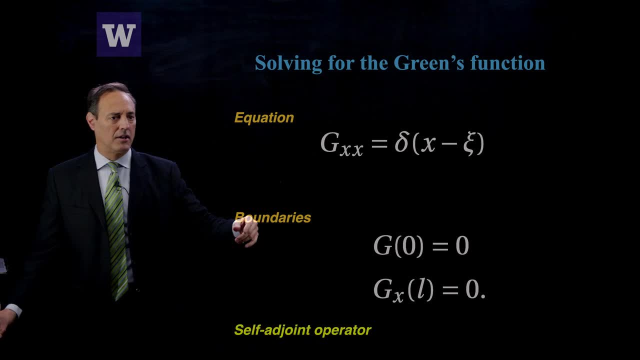 We're going to say: take this, the adjoint problem forced by the delta function. I have the same boundary conditions because it's self-adjoint. So I have to solve this set of equations to find the Green's function, And so what it is is a second-order differential operator. 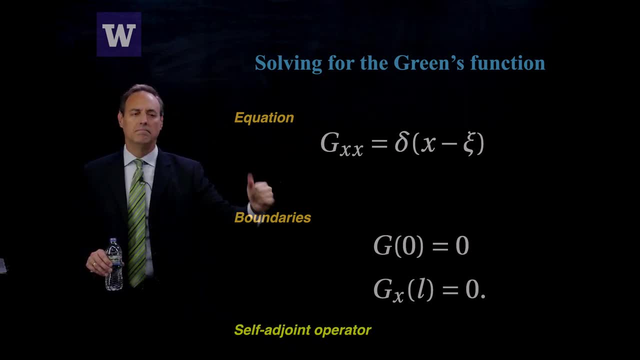 with a delta function on the right hand side. How do I handle that? We have to think about how to do that right, Because this thing is basically zero everywhere, except at x equals c, where it's a giant spike to infinity, but such that the integral area on the curve is 1,. 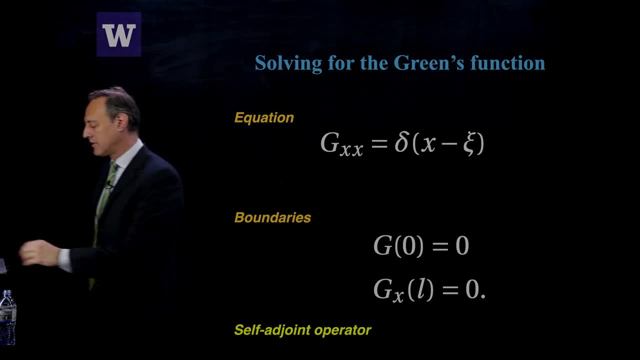 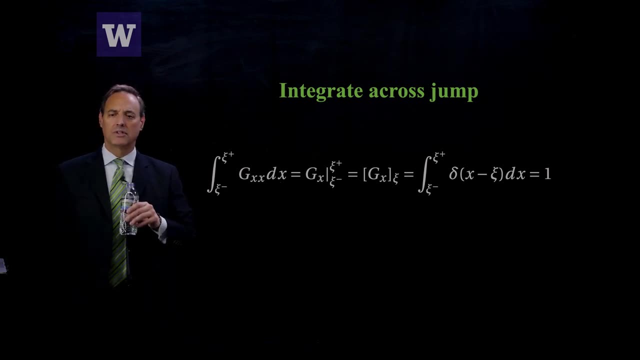 and with the boundary conditions. So let's go ahead and talk about how to solve this. So first of all, let's talk about what happens across that jump at x equals c where the forcing functioning is acting. So I take my operator. 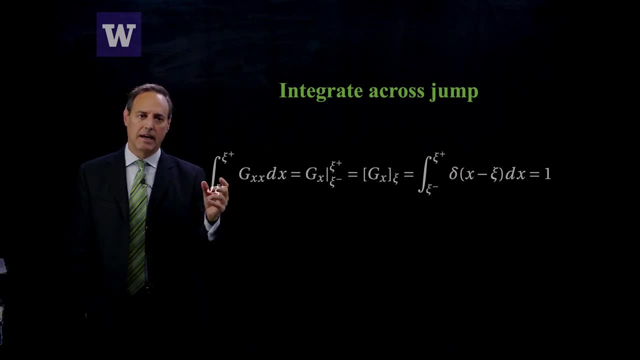 L, which is gxx. So that's the left-hand side. And I integrate across the jump from c minus to c plus, So that's the left-hand side. When I do that integral, well, it's gxx, so I integrate it once. 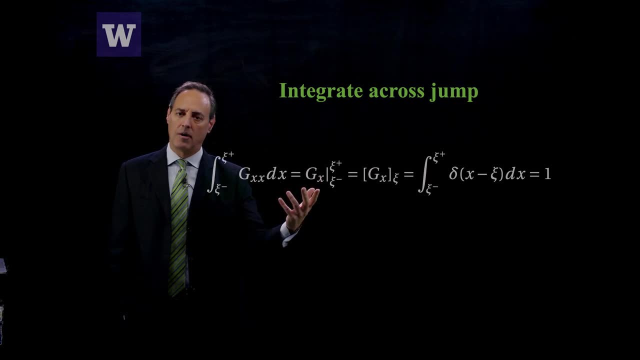 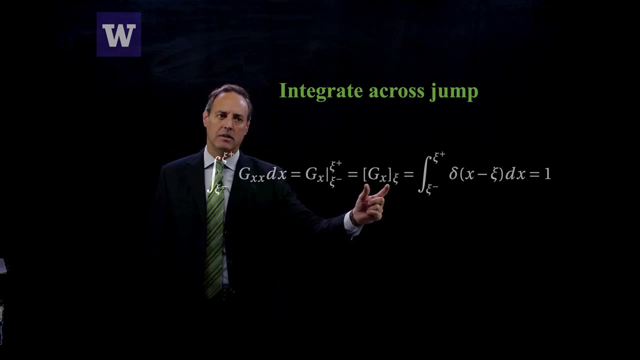 g of x, And so this is giving me then a jump in the derivative on the left, which I can represent in these square braces. g of x, c means this is the jump in the derivative. on the left side It's equal to. on the right-hand side, I have the delta function. 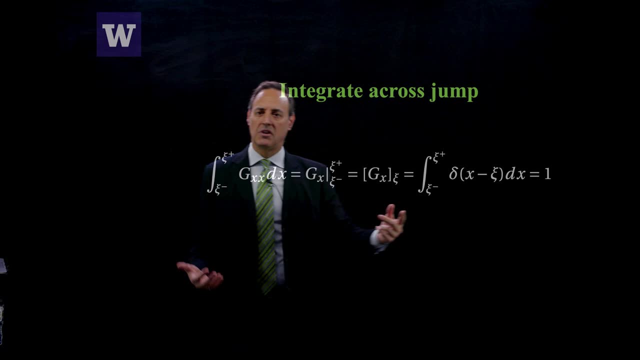 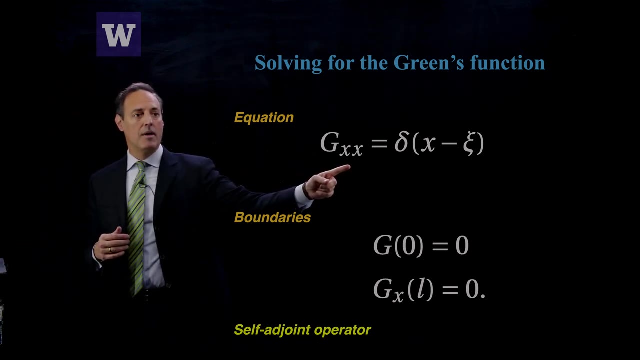 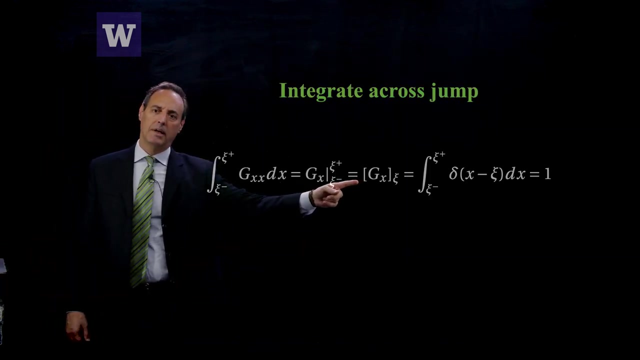 which, when I integrate it, area of the curve is 1.. That was the definition of the impulse. So what I find is, when you come back to this equation here and you integrate both sides, what you end up with is this condition here: that the jump in the derivative is equal to 1.. 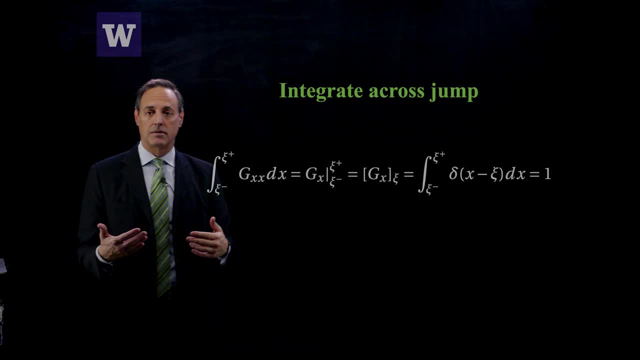 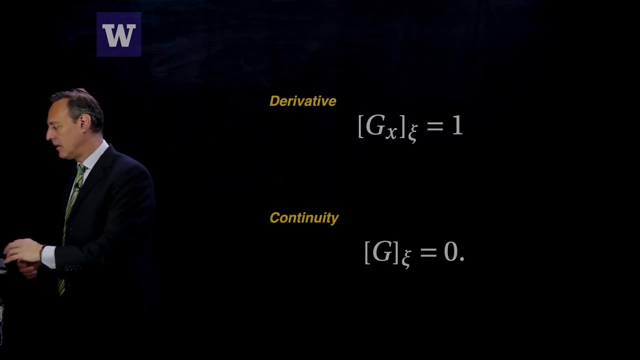 So the derivative itself is discontinuous and it has a jump of 1.. And we just calculated that. So that's what we have here: The derivative and the jump. The jump in the derivative is here. It's given 1.. 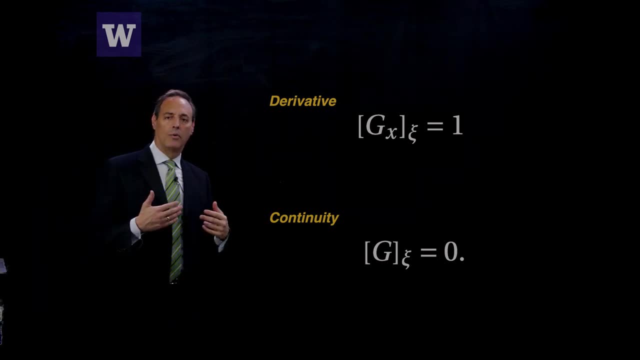 We're also going to enforce continuity. So what we're forcing continuity is we're going to say the solution is continuous, which means the jump in the solution at c is 0.. There is no jump, It's continuous. So these are going to be two constraints we place on the Green's function. 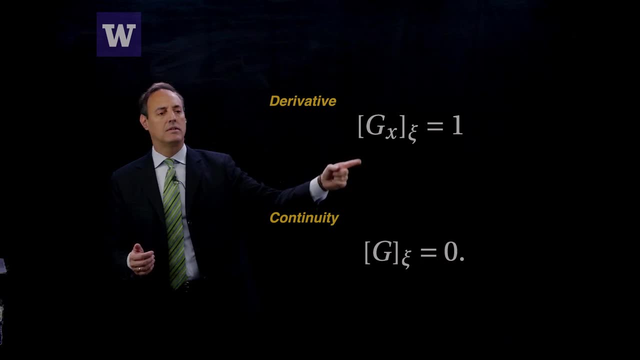 Okay, So the first one just comes from integrating both sides. The second one comes from this is: we're going to assume that we have that the Green's function is going to be a continuous function and those are going to be two constraints we have to impose on this to find the Green's function. 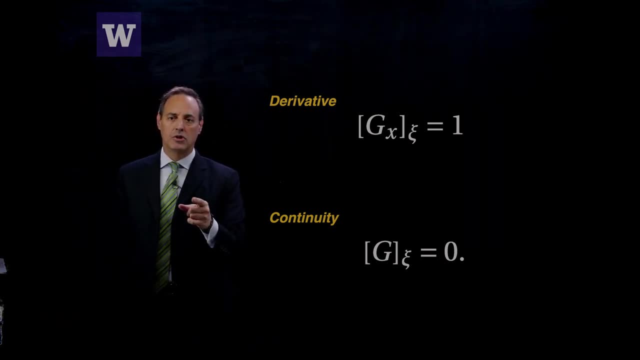 But that answers the question of what happens when I have this giant delta function sitting there on the right-hand side. right, It's 0 everywhere, and then it goes to infinity at one spot. What does it do? It does exactly this. 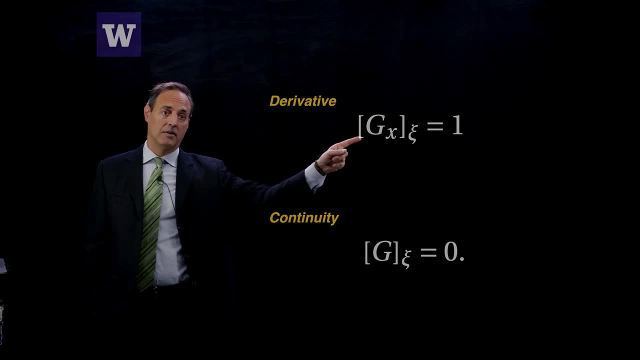 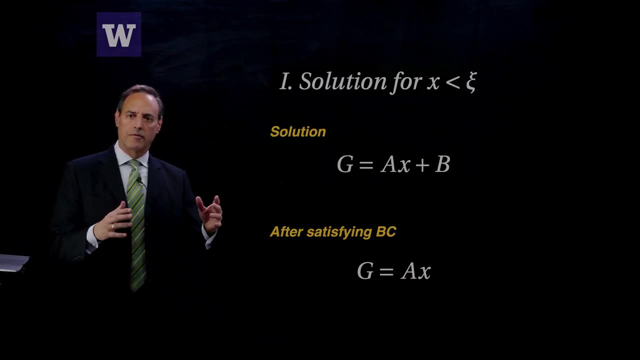 This is the consequences of it. It creates a discontinuity in the derivative, but the solution itself will be continuous, The solutions by the way to this. then we solve it for the left and the right of the domain, If x sorry, left or right of where the forcing function is acting. so for x less than the c. 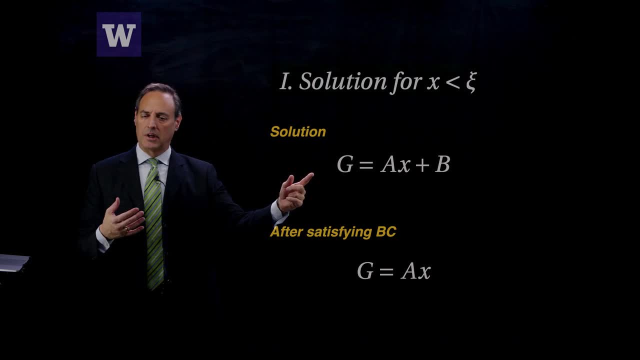 you have a linear solution: ax plus b, because this is just a second-order operator. gxx equals 0. You set the boundary condition into it and it just takes: makes b equals to 0, so it gives you a solution ax. 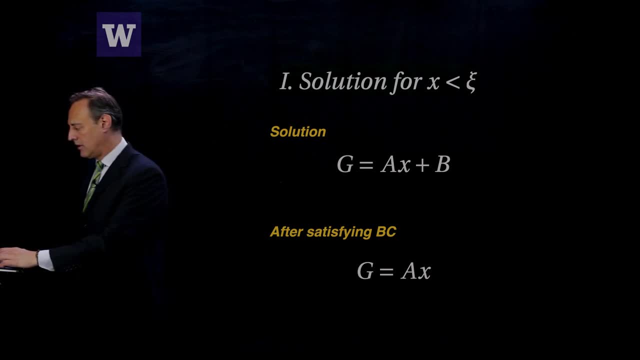 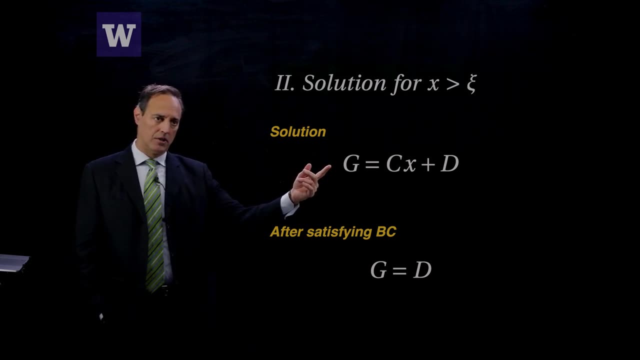 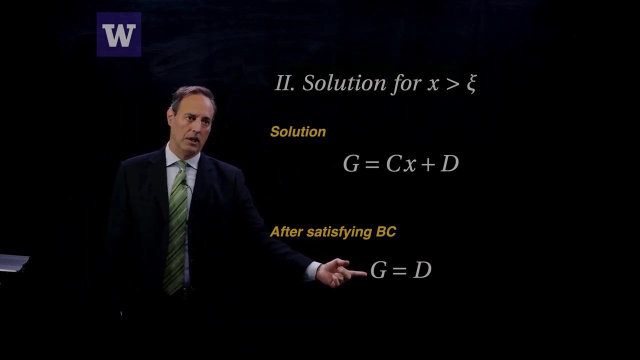 So that's the solution to the left of this function, The solution to the right same thing: A linear equate, a linear relation like this: cx plus d. Set the boundary condition into it and you find that in fact, g is equal to d. 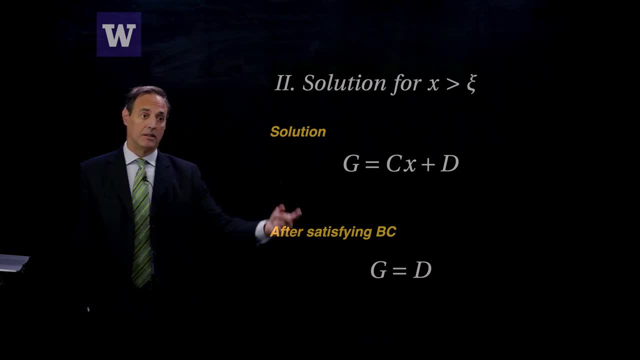 because the derivative has to be 0 at that boundary, making c equals 0.. So now you have this constant as a solution. so in fact, on the left and the right each have an arbitrary constant. but now that's two unknowns, but you have two equations left to enforce, which is at the jump. 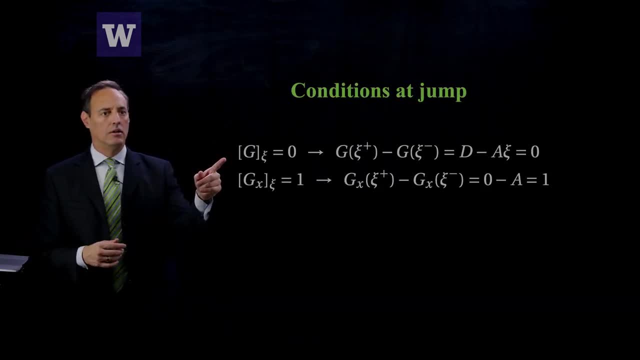 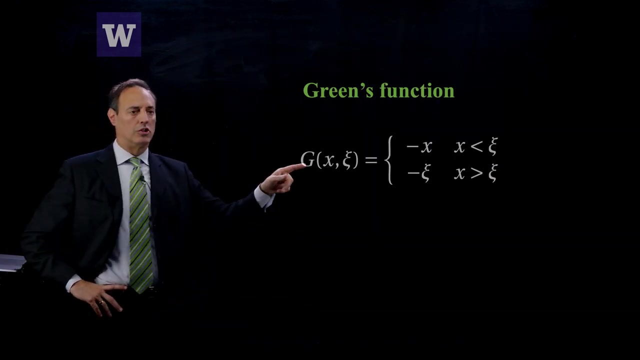 you have continuity right here and you also have the jump in the derivative is 1. If you impose both of those, it gives you two equations for two unknowns that you have left still into that problem, And then that uniquely then determines the Green's function which is given right by here. 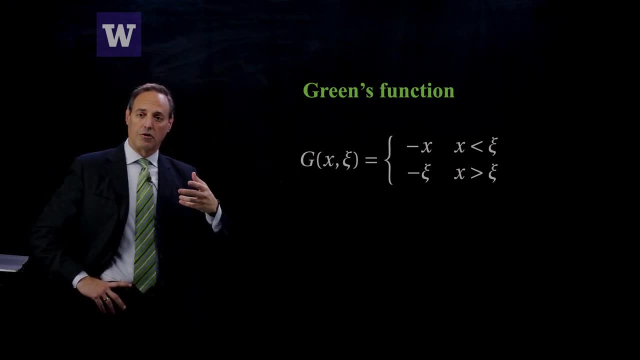 Okay, So The Green's function is broken down to two parts: to the left of the delta function, to the right of the delta function, and there are the solutions. Notice how it's symmetric. If you were to place interchange x and xi, which we will do, 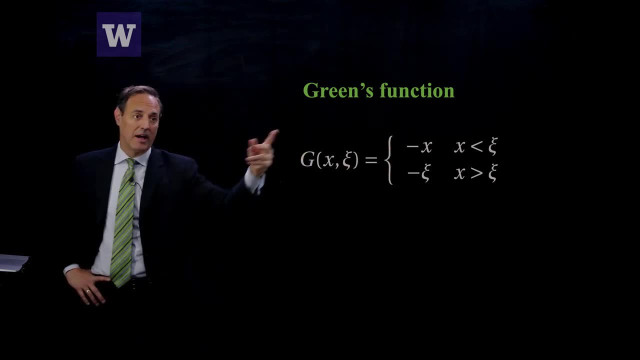 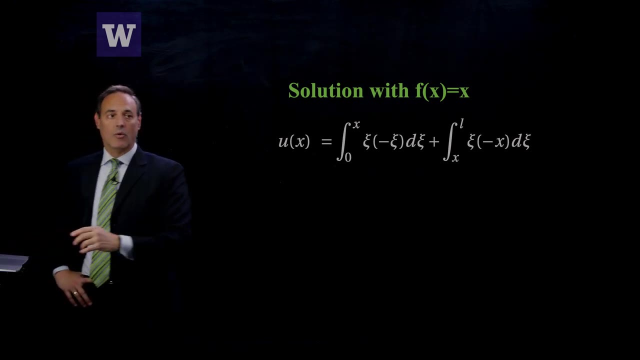 then these here just interchange And x becomes xi, xi becomes x and it's symmetric with respect to those two variables. So if we had put in our solution originally which is f of x equal to x, then all we have to do 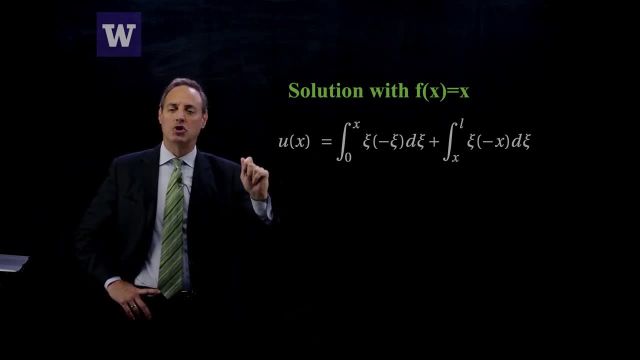 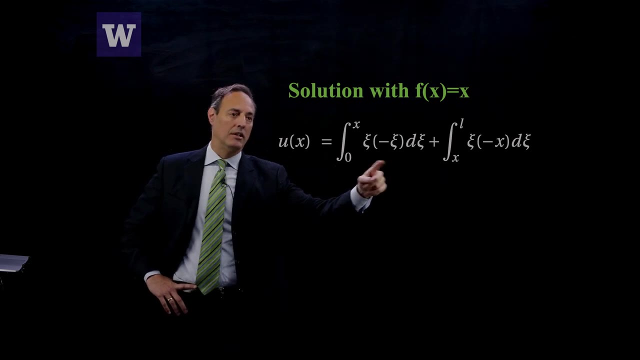 is. take this: u of x is equal to now. I take g of xi of x, not x of xi, integrate against f of xi and what you find is if you break this down now, it becomes integral from 0 to x and x to l. 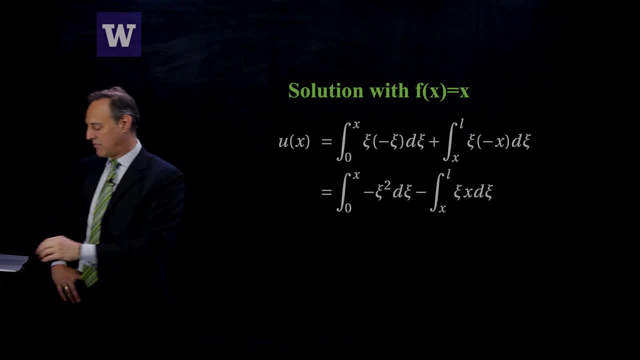 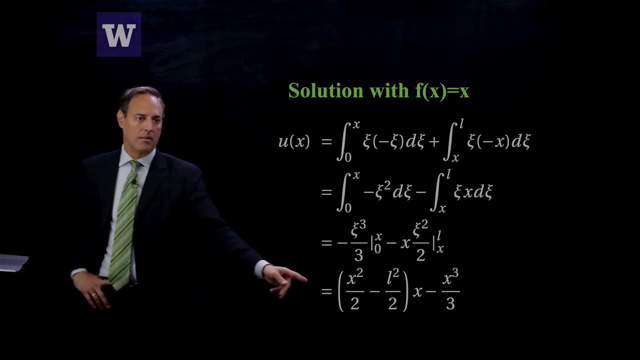 Integrate both of these here and then. so this integral is actually pretty simple to do. There you go, evaluate at the limits, and there is your solution to the problem right there. So now we have this solution And we're going to do the same thing. 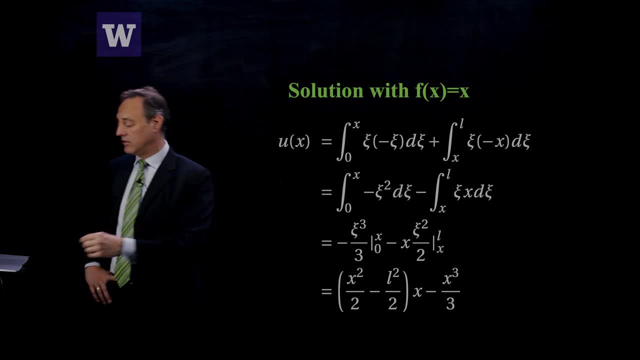 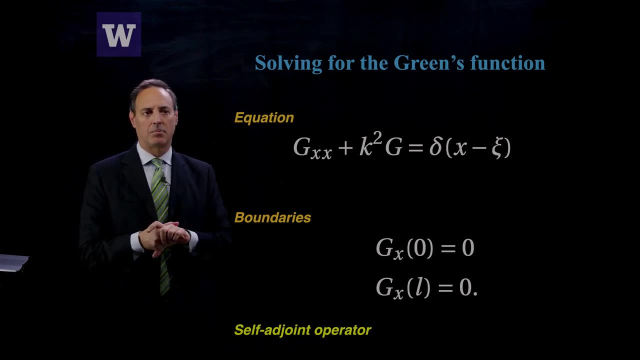 for that function, of that problem given by solving this using the Green's function. Let's do one more example. Second example I want to do is this one: here, g of x plus k, squared g, is equal to the delta function, And all I'm going to do here is compute the delta function. 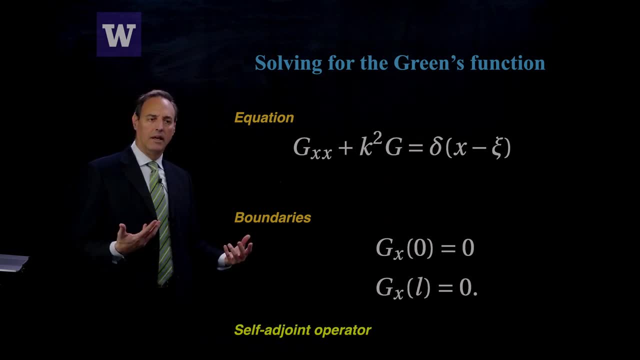 And here are the boundary conditions: No flux. Now, this is coming from a self-adjoint operator, So if you had l equal to f, it would take very much the same form, but you have an f over there on the right-hand side. 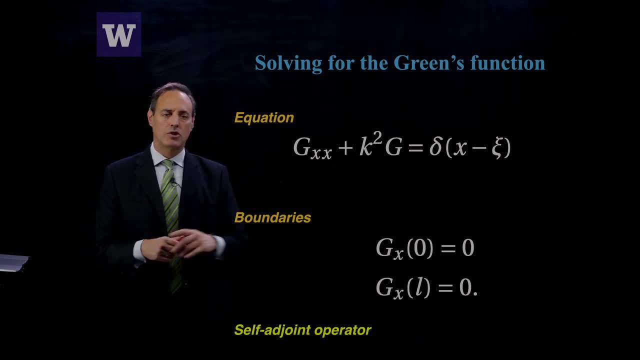 But I just want to construct the Green's function for this. And so again we're going to say: delta is equal to 0 everywhere except at c, And so I want to solve this to the left and to the right, which means g of x plus k squared, g is equal to 0.. 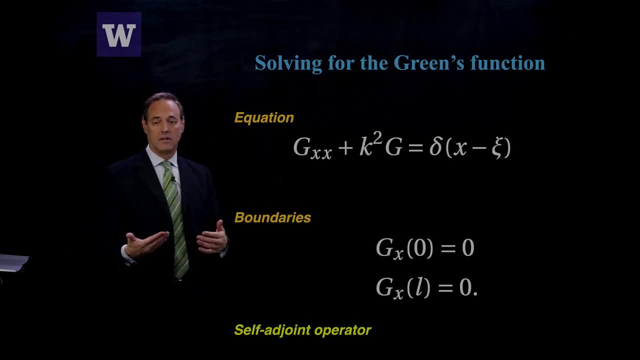 The solutions to that are sines and cosines. And notice: I have no flux boundary conditions at 0 and at l, So the only thing that's going to satisfy these is cosines. Sines will violate these, So I'm going to have cosines. but now I'm 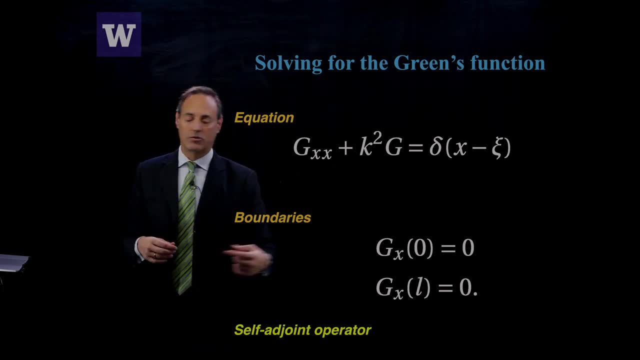 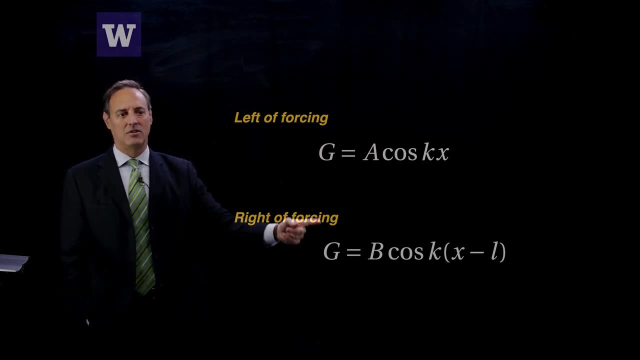 going to have a cosine centered at l and a cosine centered at 0 to do it. So, in other words, I can rewrite this as the solutions like this: g is equal to a cosine kx, g is equal to b cosine kx minus l. 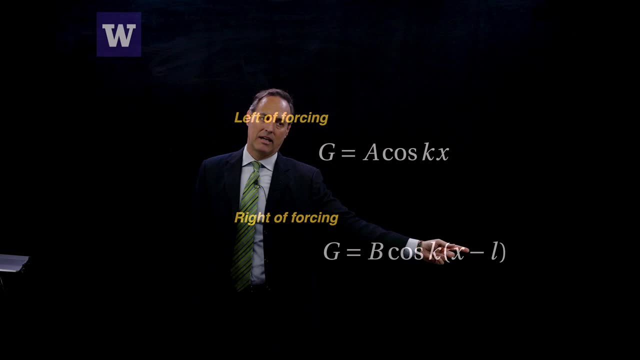 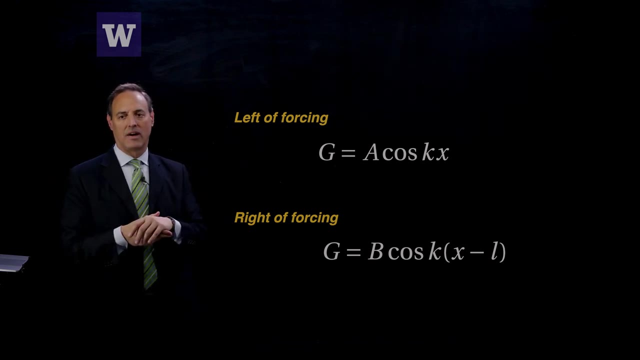 Again, the reason I've centered this at x minus l is because when you take the derivative of that there I'm just getting, the cosine automatically satisfies that no flux boundary condition. So it's a nice little trick to use and often used in constructing these Green's functions. 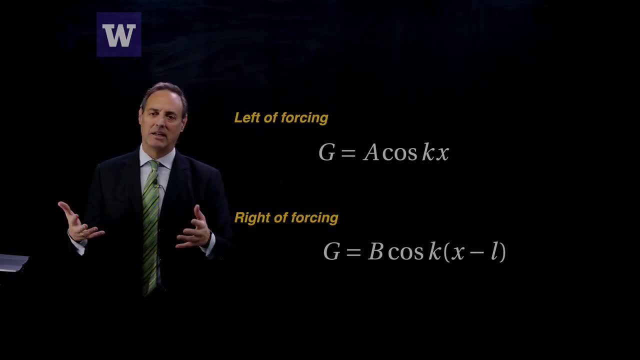 You recenter some of these functions to make it easier to do manipulations with. So these are like pro-level tips, by the way, for solving these kind of equations. This is what everybody does, Those who are in the know. this is what they do. 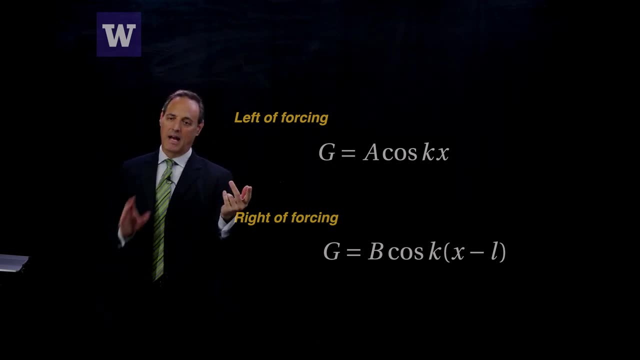 And so, notice though I have these constants a and b still unknown, but I haven't satisfied yet the jump condition around continuity or the jump in the derivative conditions. So When I apply those, I'm going to get two equations, two unknowns for a and b. 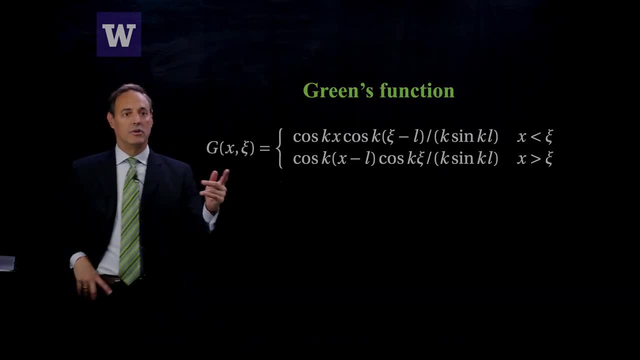 I can solve for those and I find the Green's function. Here it is. Here is the Green's function written all out. And notice again, it's symmetric with respect to x and xi. So I can reverse these, which I do when I do the integral. 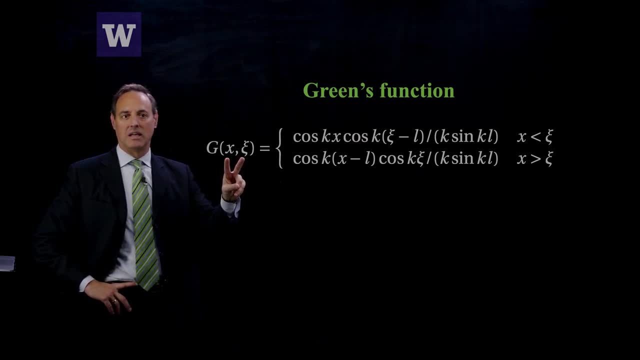 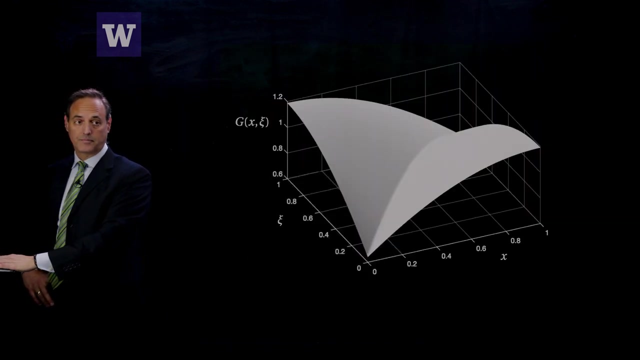 Instead of integrating g against x comma xi, I actually integrate gx comma x. These are just dummy variables, So you can just change where the x and the xi are and then we're going to integrate that to get fundamental solutions or to get a solution. 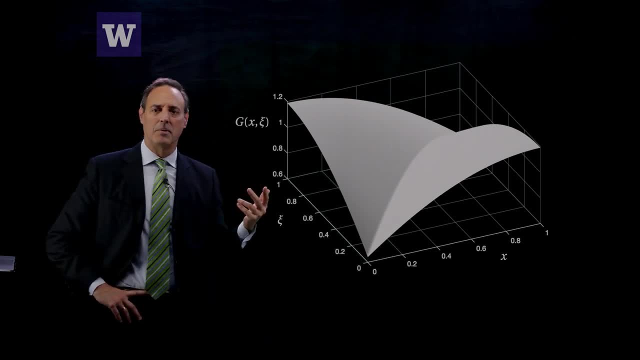 And, by the way, I also wanted to plot what the Green's function looks like. A lot of times people don't plot these Green's functions, but here it is. So here is the xi axis, the x-axis, and here's what the Green's function looks like. 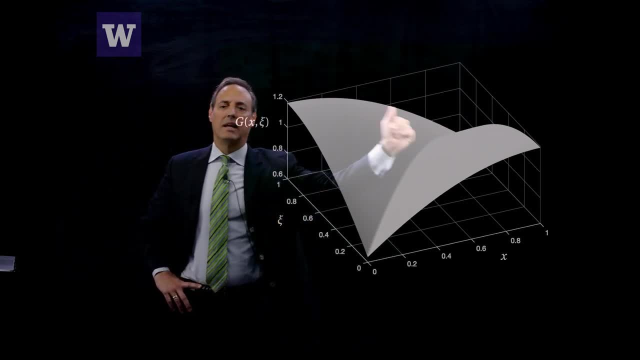 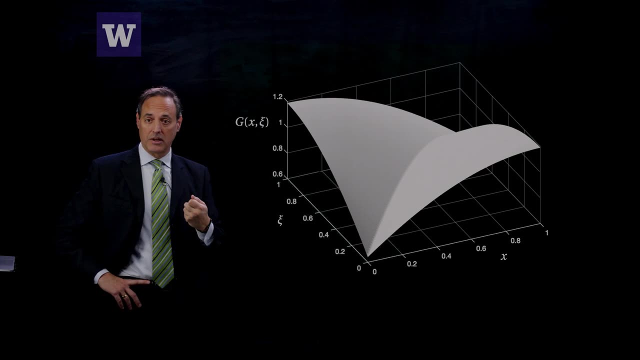 And notice this diagonal line running down the middle of this thing. that's x equal to xi, In other words, where the delta function is acting. And, of course, what you expect there? well, you expect the solution to be continuous, but there to be a jump in the derivative which 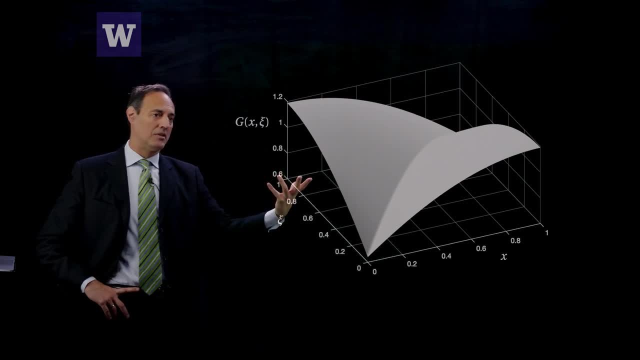 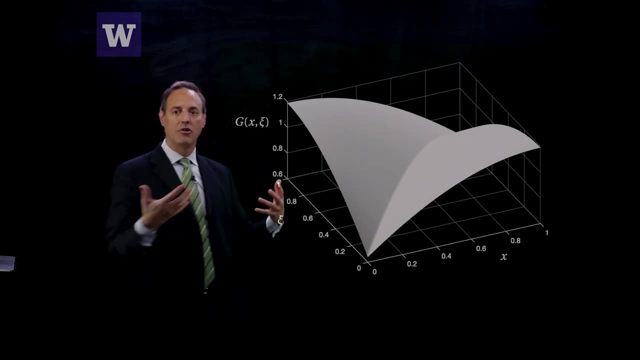 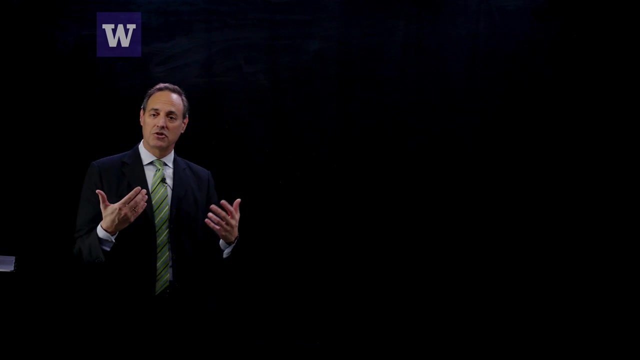 is exactly what you see there. So this is a nice representation of the Green's function. And you give me an f of x, you integrate it against this Green's function and you find your solution. So there you go. That's the introduction to the Green's function.